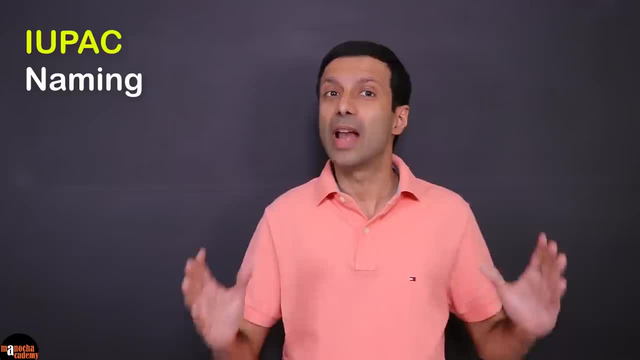 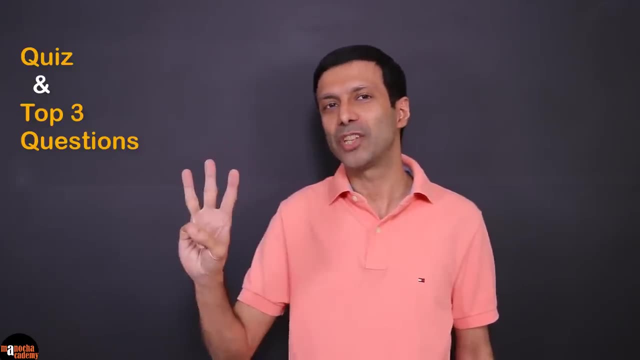 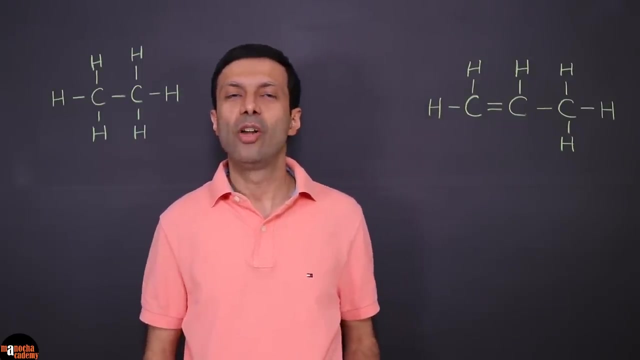 as easy as writing your own name And if you like this video, do share it out with your friends And don't forget to try the quiz and the top three questions on this topic. Links are given below the video. There are some important rules that we need to follow for IUPAC naming. I'll 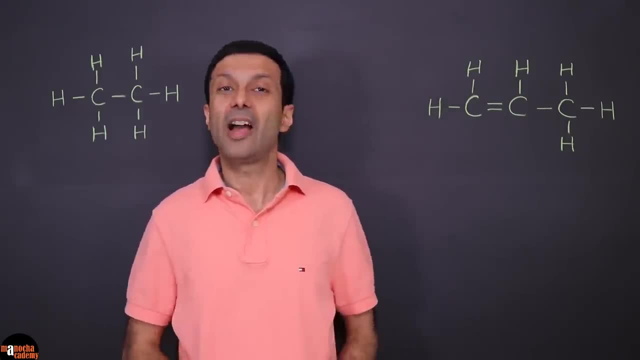 show you the rules with the help of some examples. I recommend you to sit with a pen and paper, So let's go ahead and do this IUPAC naming together. Let's start with this simple example. So what do we have here? 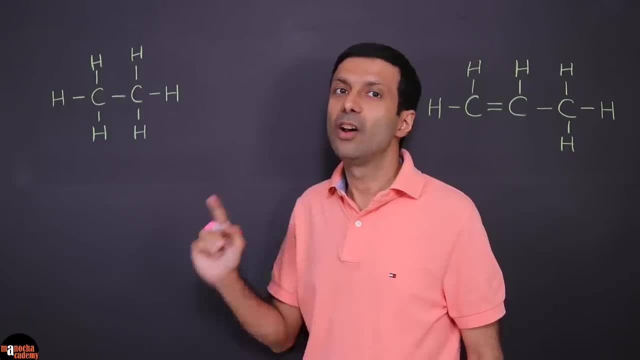 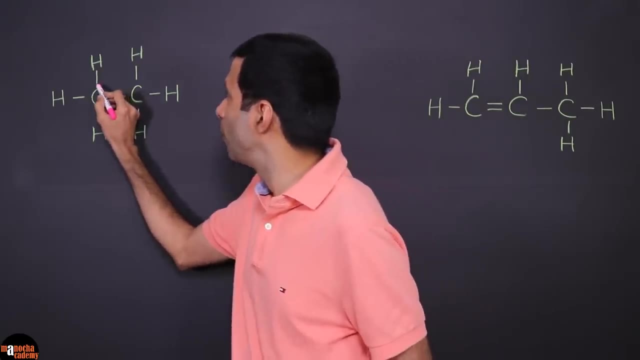 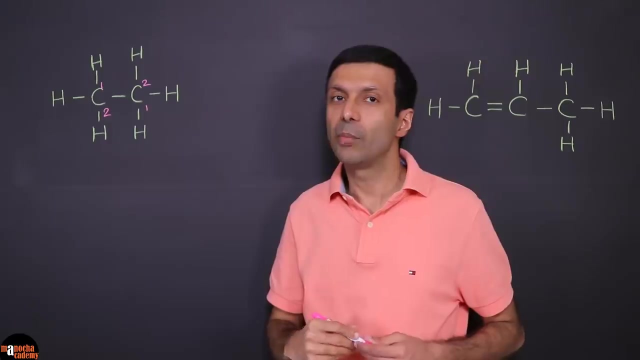 To name this compound, you need to first find the longest continuous carbon chain, which is this: two carbons here. Now go ahead and number it forward and backward. Now why do we do the backward numbering? We'll discuss that later in the video. 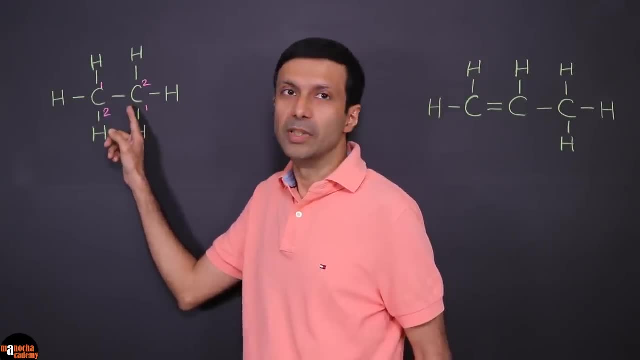 As you can see, this compound has two carbons. So what is its name going to be? Remember, there's a table, if there's one and then the other. So let's say there's a 12.. Now let's say there's a 12 and then there's a 13.. So let's say there's a 13.. 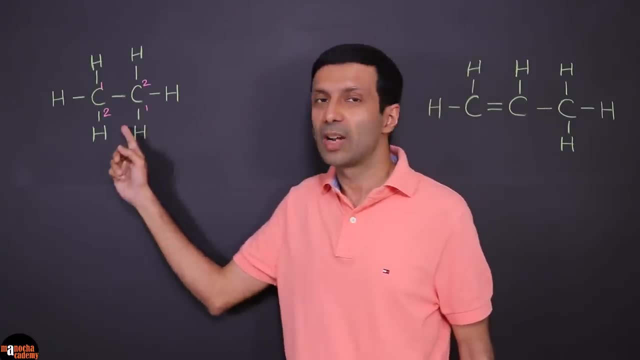 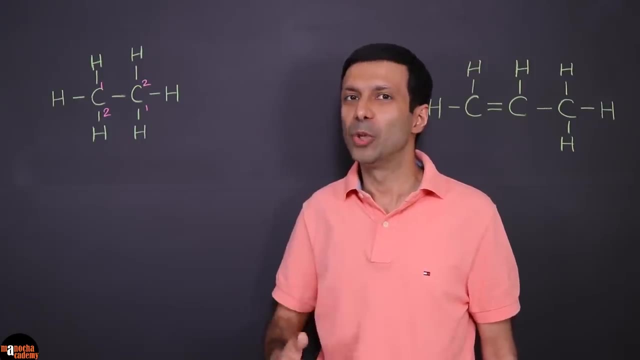 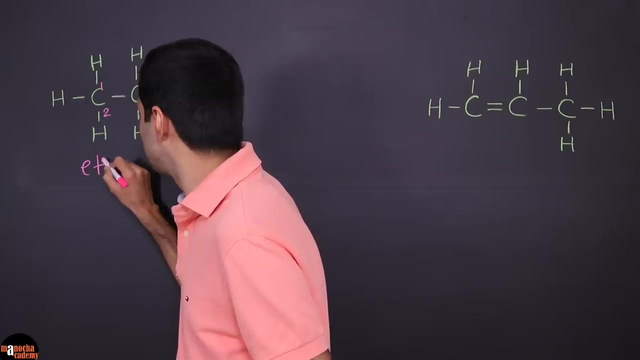 one carbon. then the name starts with meth. Two carbons. the name starts with eth- Three carbons. it will start with prop. Four carbons, bute, and so on. So the name of this compound will start with eth. And what type of bonds are there in this hydrocarbon? So you need 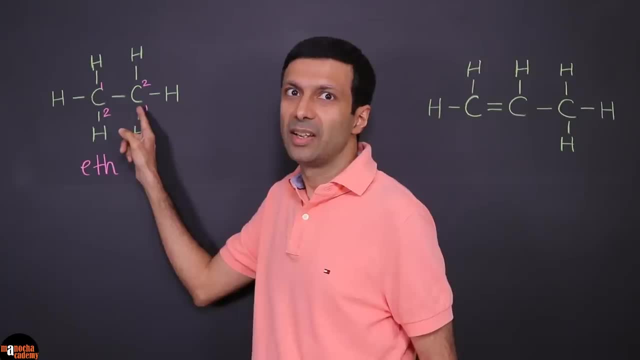 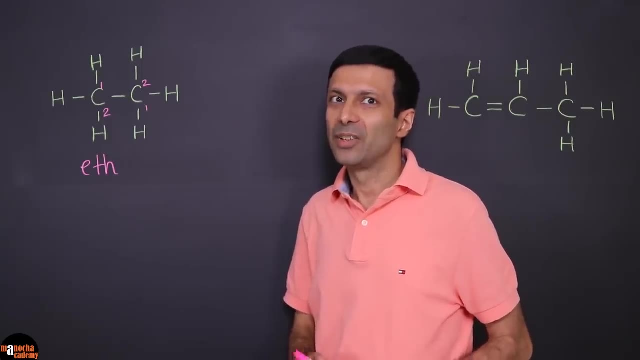 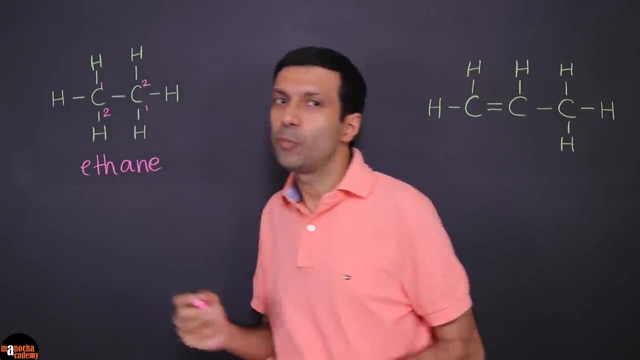 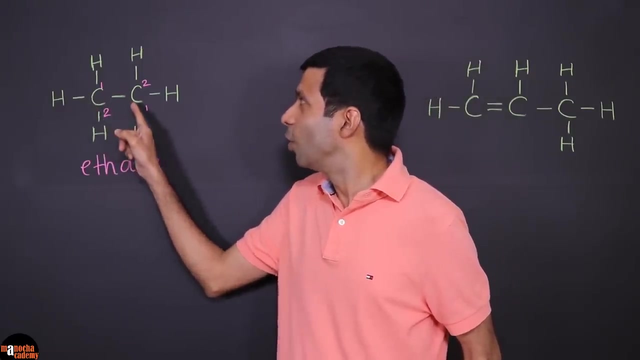 to look at the bonds between the carbon atoms And, as you can see, there's only a single bond here. So this hydrocarbon is an alkane, So the name will be ethane. So that is the IUPAC name of this compound. It's ethane. So what did we have to do? Look for the longest. 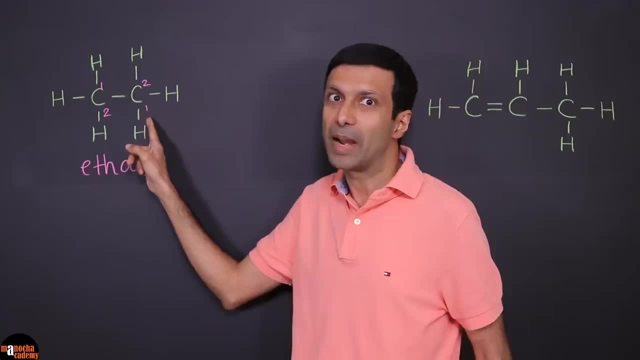 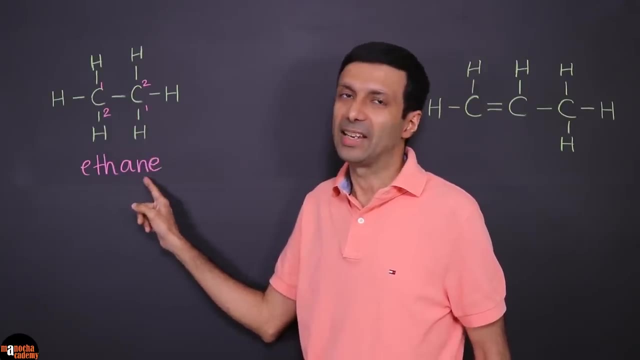 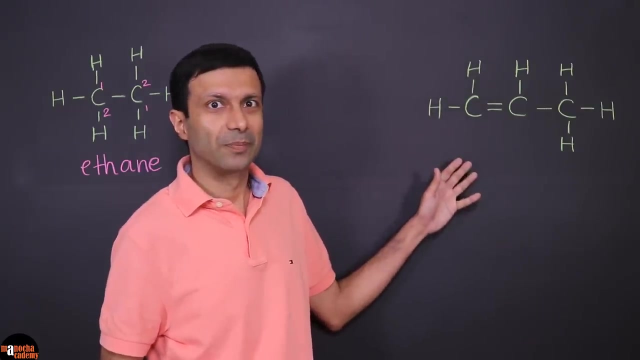 carbon, continuous carbon chain. number it forward and backwards and find the longest one And the name based on it. it was eth, And since they are only single bonds, it's an alkane, So it's going to be ethane. Now let's go ahead and take a look at this example. 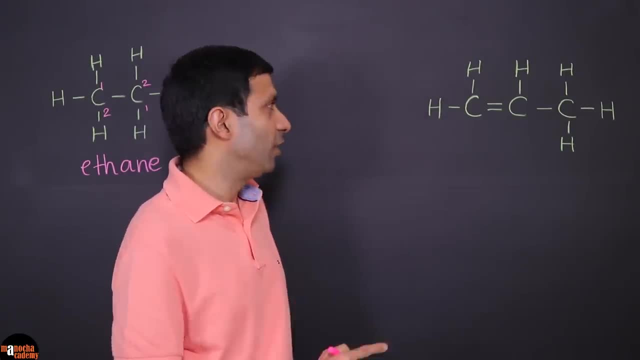 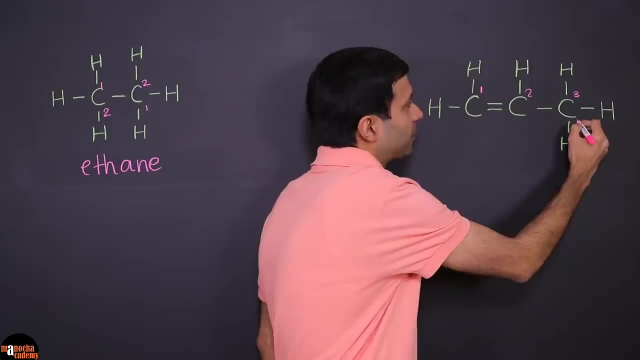 So let's apply the same rules. We are going to find the longest continuous carbon chain, which are these three carbons, and we'll number it forward and backwards. So three carbons means the name is going to start with eth And the name based on it, it was eth And since they are only single bonds. it's an alkane, So it's going to be ethane. Now let's go ahead and see if we can find the second compound. So we would take the another compound. So let's take one compound and say that this compound is a propane, So the compound that 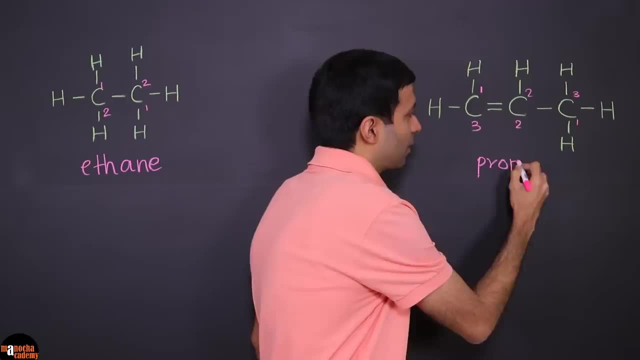 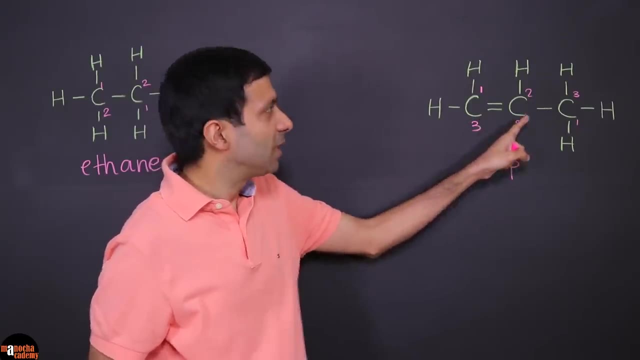 we were talking about will form a single bond, a single bond. The second compound: this is a propane. That's right, prop. And is this a propane? No, Because there's a double bond here. So there's a single bond between these two carbon atoms, but there's a double bond. 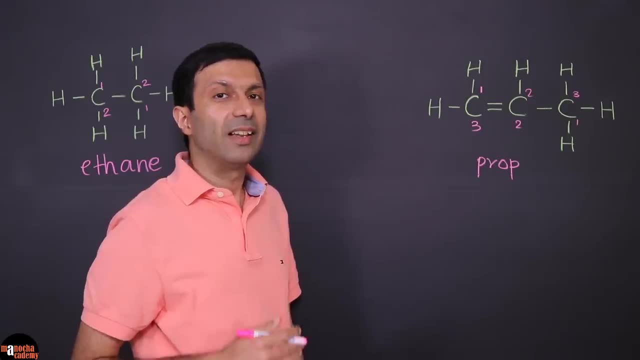 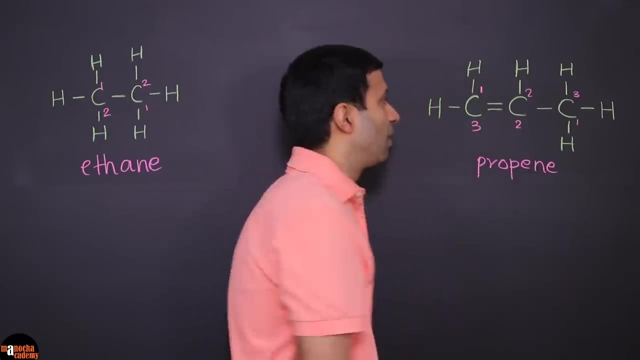 between these two carbon atoms. So it's an alkene. So the name is going to be prop-ene. And if we had a triple bond here instead of a double bond, how would we find this? We could find it by making this a triple bond, So you can call it an alkene. Now, if we had 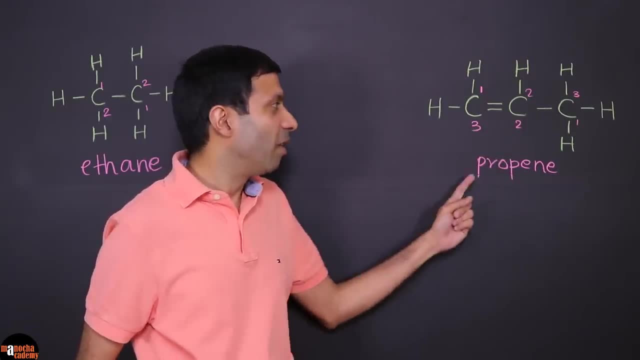 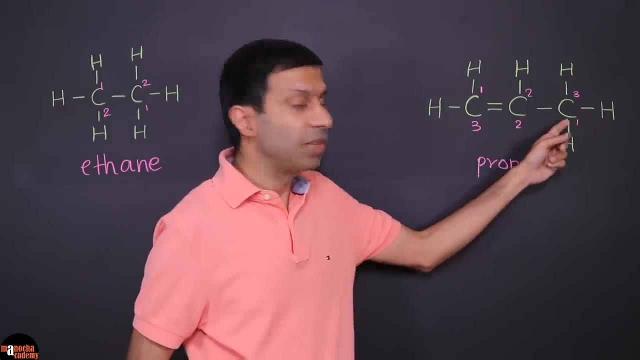 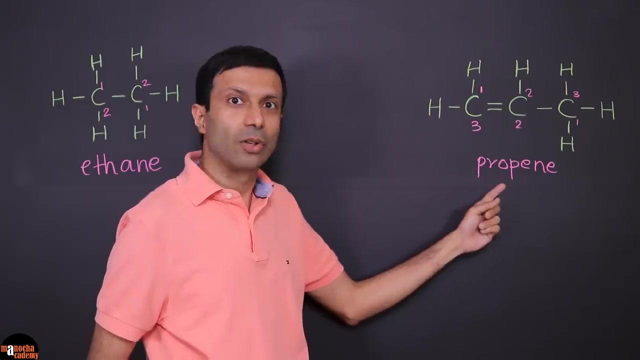 bond. what will the name be? that's right. it would have been prop ion. okay, so what we learned here is that you need to look at the longest continuous carbon chain, look at the number of carbon atoms. once you've numbered it forward and backward, find the name based on the number of carbon atoms. 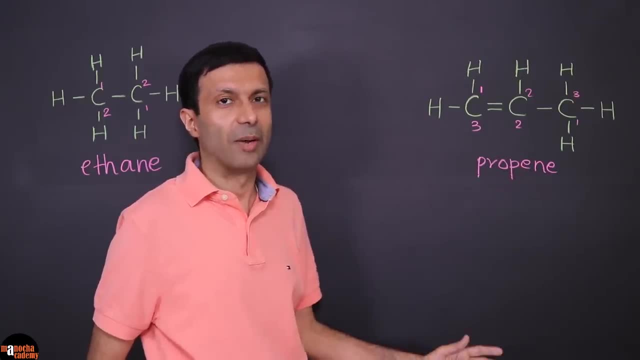 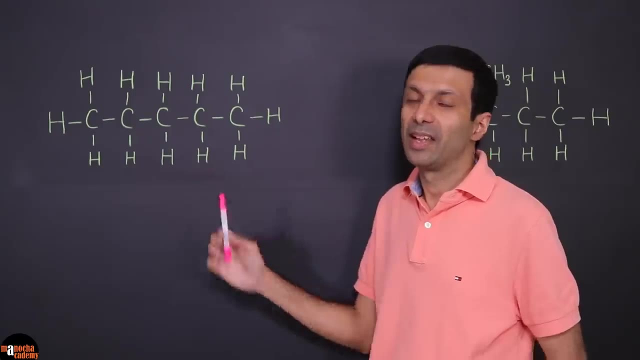 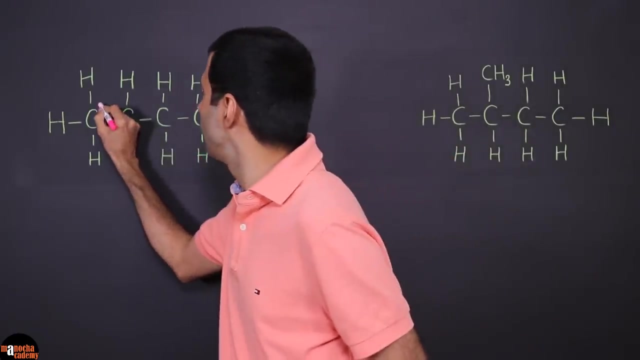 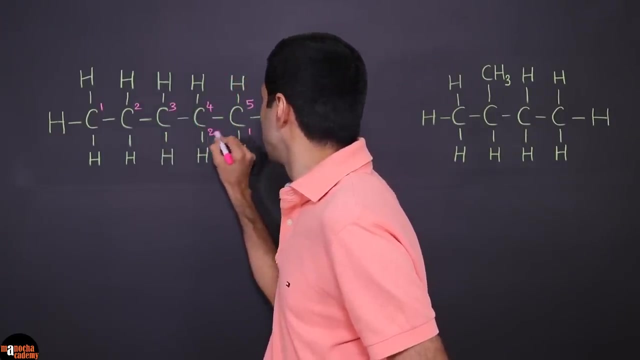 and also the type of bond for these hydrocarbons. let's take a look at this example. what will be the iupac name of this compound? again, let's find the longest continuous carbon chain, which is this one, and let's number it forward and backwards, so it's a five carbon chain and we are going to do. 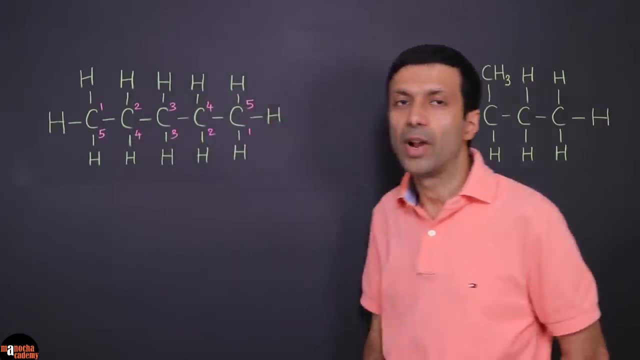 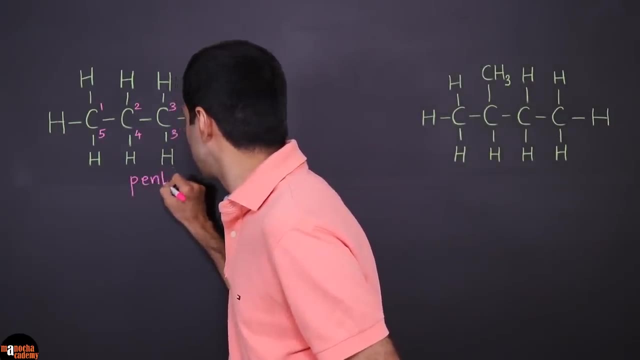 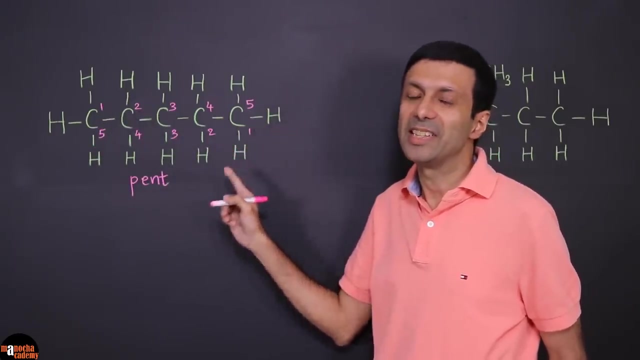 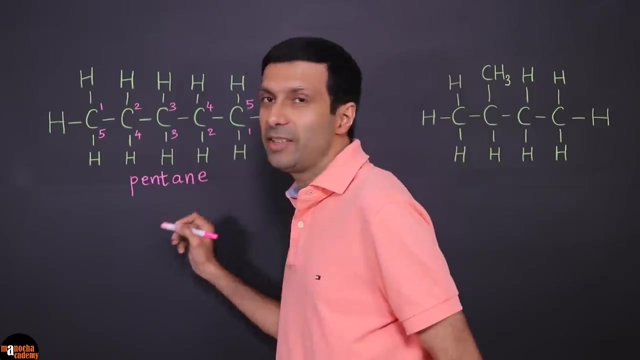 the forward and backward numbering. so five carbon means the name is going to start with pent right, and since there are only single, single bonds between the carbon atoms, this is an alkane. so what is the name? it's going to be pentane right. so this is a simple one. but 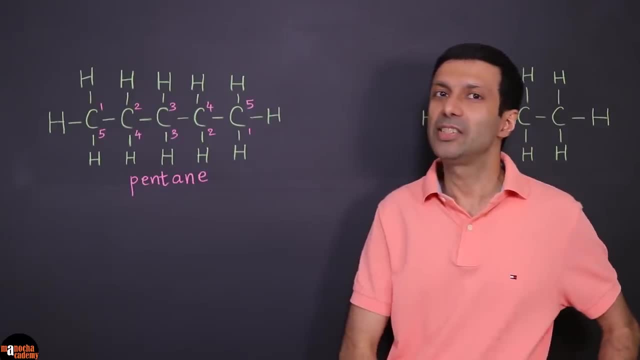 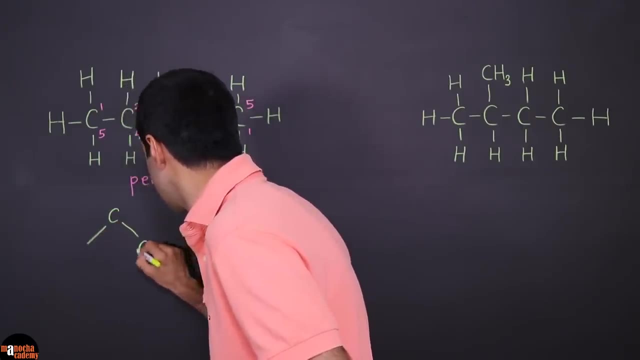 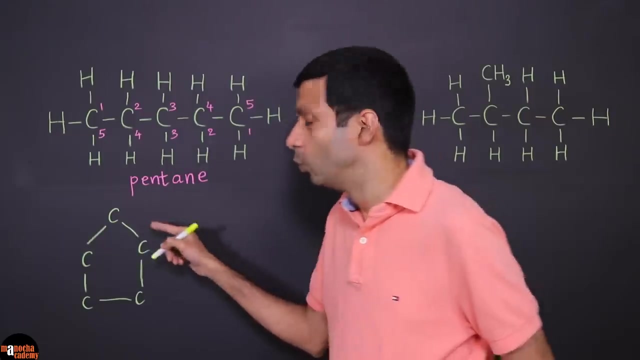 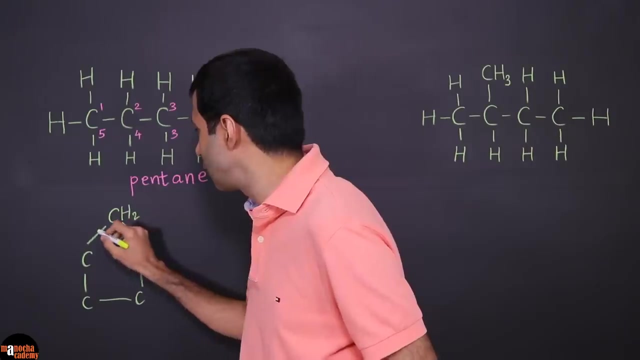 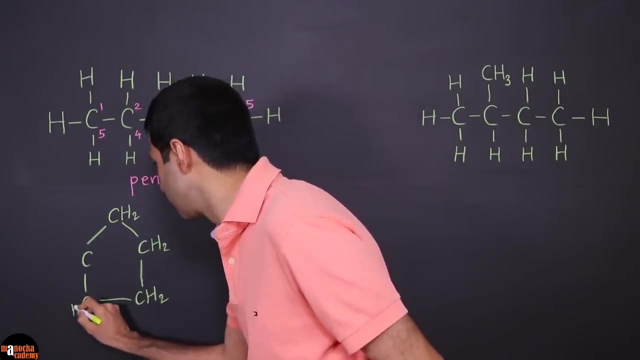 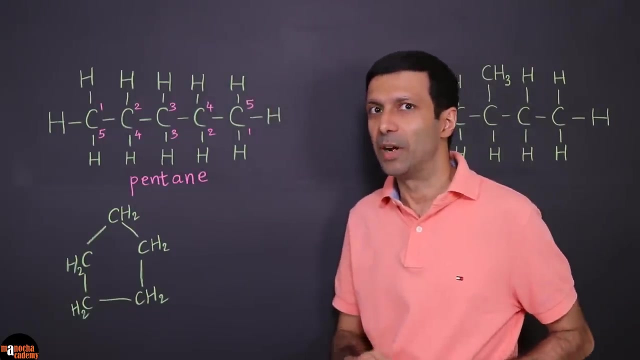 now, let's say the five carbon atoms are arranged in a cyclic structure, something like this: and to fill in the, let's fill in the hydrogens, so that carbon has all the four bonds satisfied. so one, two and two hydrogens. same way here. so what will be the name of this cyclic compound? so the cyclic compound. the name starts with the. 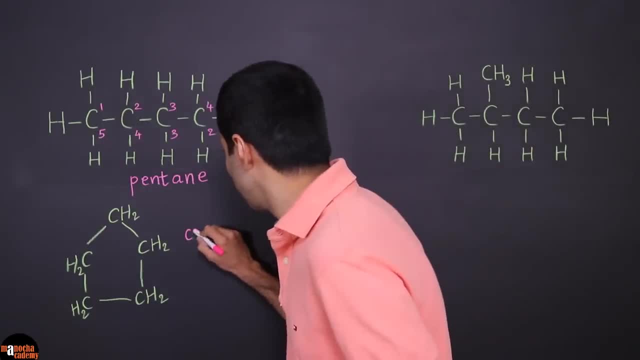 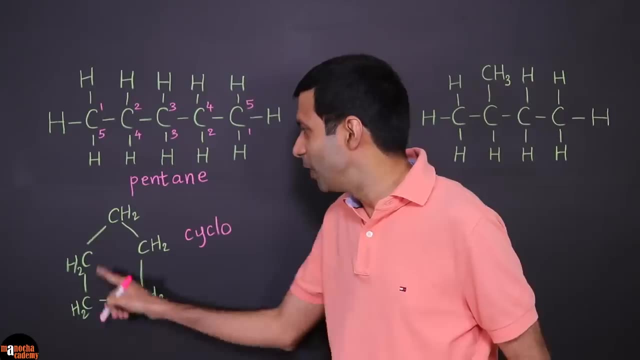 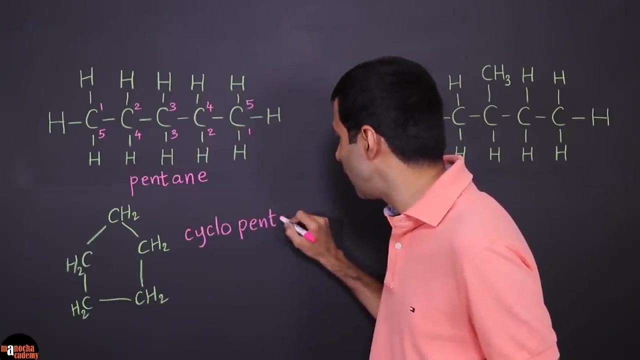 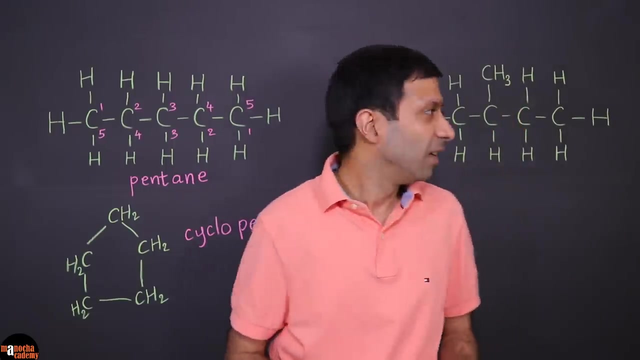 word cyclo. so remember it's going to be cyclo, not psycho. and since there are five carbon atoms, here again it's going to be cyclopentane, pent, because five carbon atoms and only single bonds, so it's a cyclopentane. now let's take a look at this compound. so this also has five carbon atoms, but 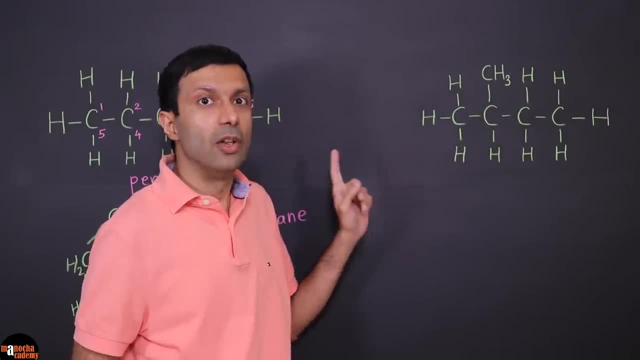 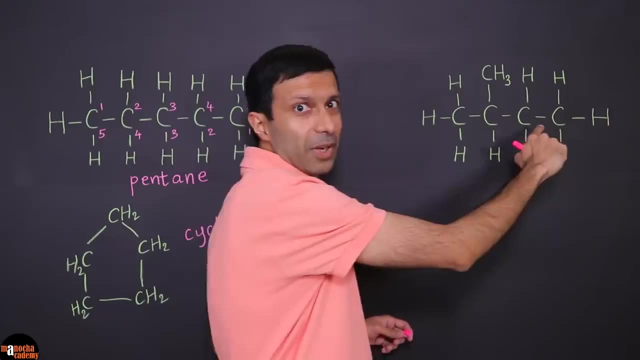 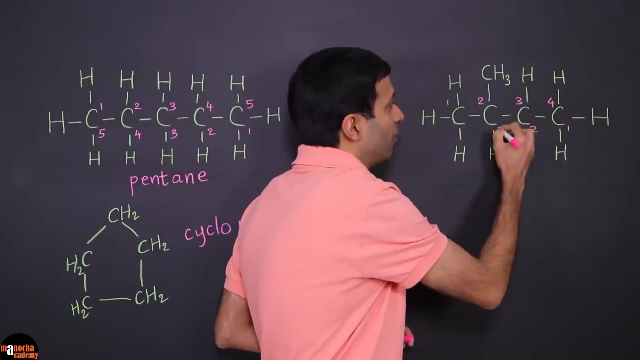 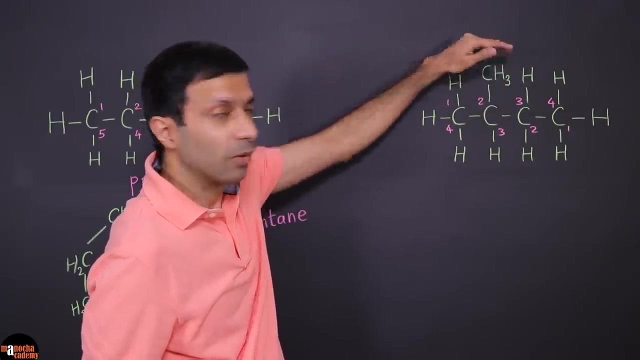 remember, we need to find the length of the bond. so this is going to be the longest continuous carbon chain, so it's going to be this one. you can't go up like this and come down, so let's number the longest continuous carbon chain and, as you can see, there are four carbon atoms here. so if we ignore this attachment of ch3 for 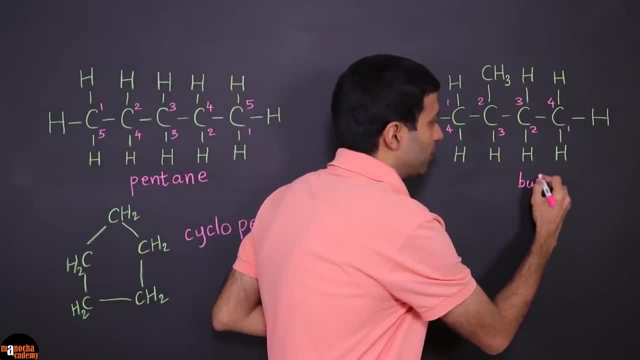 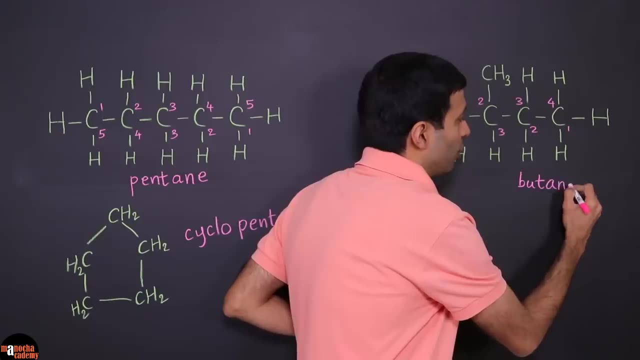 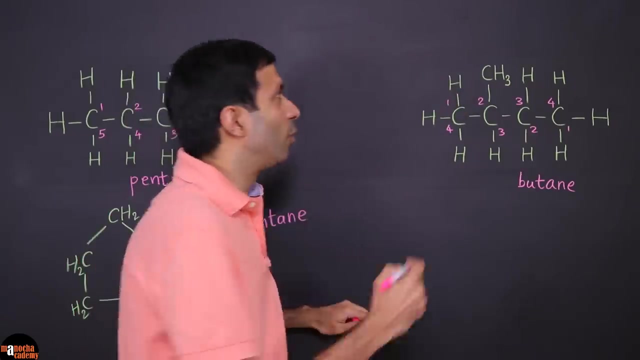 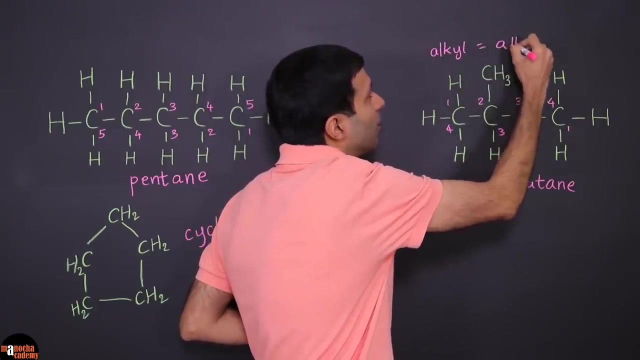 a moment. what's the name going to be? four carbon means it's going to be butte and since there are five carbon atoms, it's a butane. so that's simple. now let's look at this ch3. so ch3, as you may know, is an alkyl, because the definition of alkyl is: it's an alkane minus. one hydrogen. so if this had been ch4. but we've removed the hydrogen so we have ch3. so if it was a ch4 the name would have been methane- one carbon atom right. but this will be now called methyl right because it's an alkyl and the alkyl name comes in the prefix, so you have to put it. 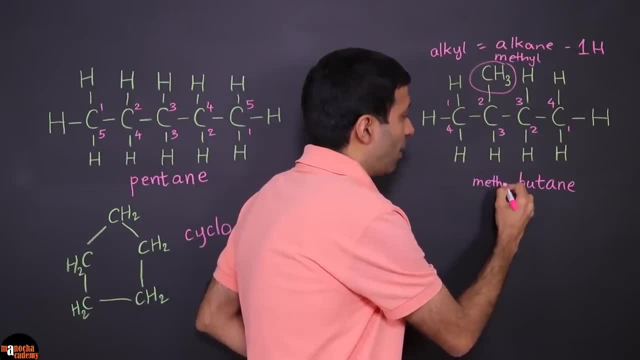 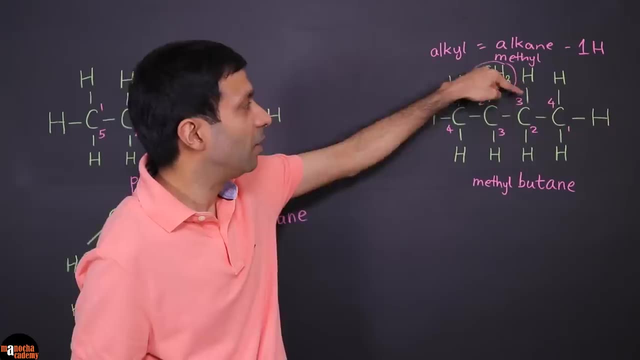 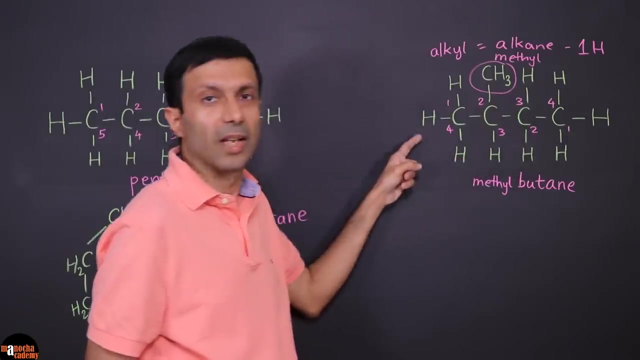 over here in the beginning of this name. so we have basically a methyl butane here, but now this methyl could have been here, or it could have been here or here. so we also need to give its position and the position is based on this numbering that we have done. so what number should 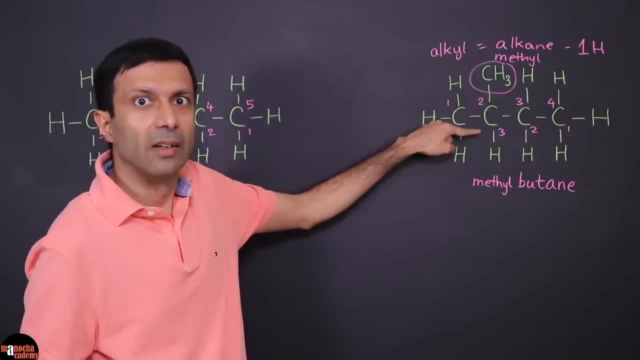 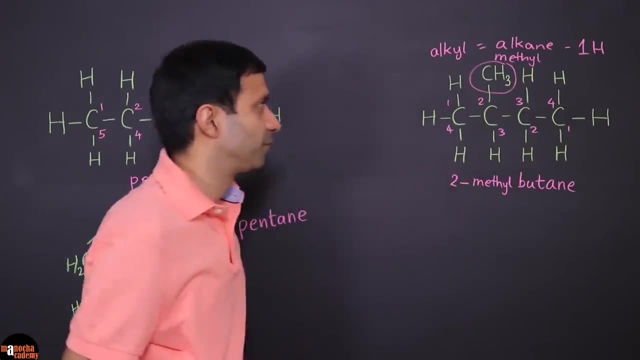 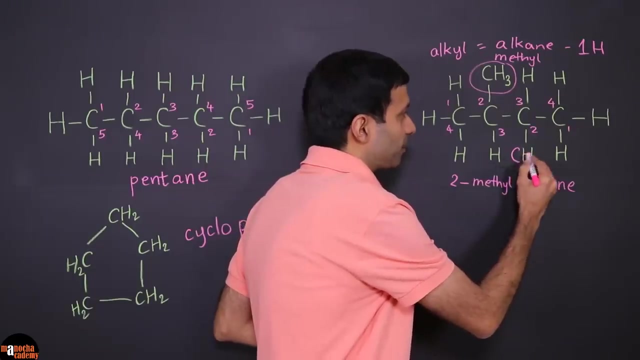 we give it. it's on number two or three, but you need to choose the smallest number. so it's going to be two methyl butane. okay, so that's the name of this compound, but let's say we had another ch3 over here, so can you guess what will be the name here? so let's work it out again. 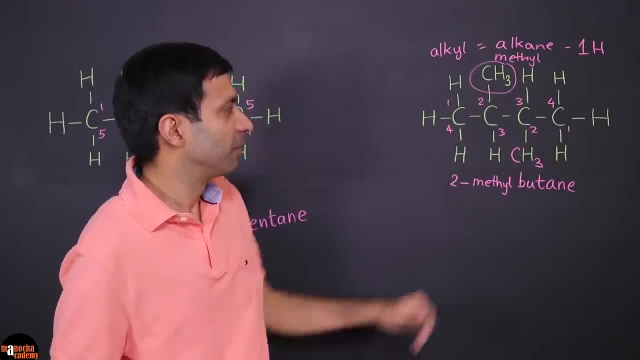 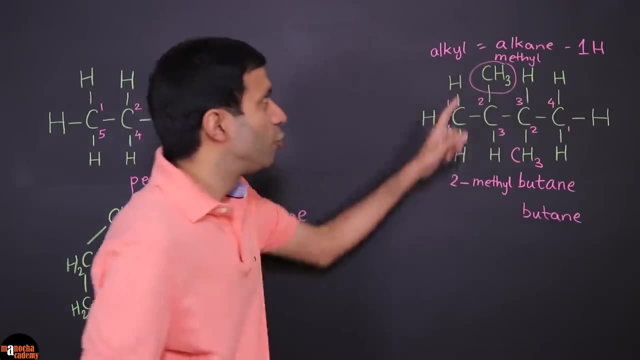 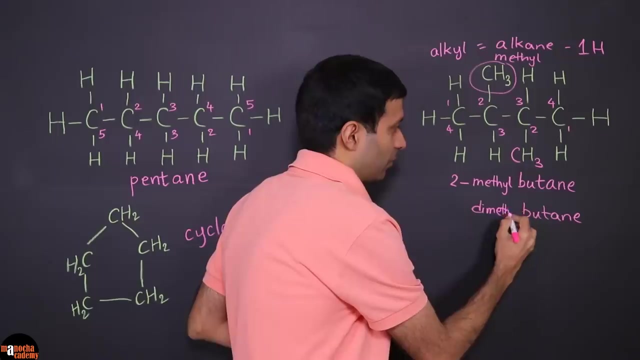 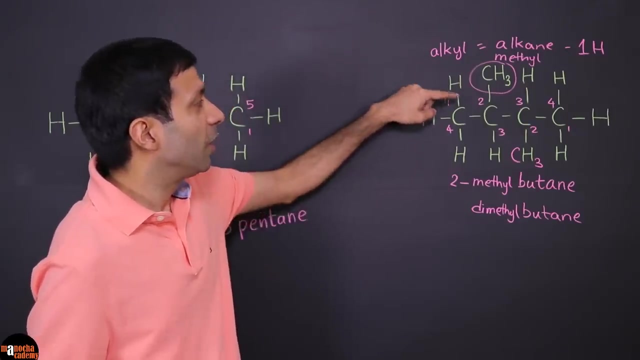 first, the trick is ignore these attachments. so it's basically a butane and we have two methyls in here, so that's going to be a dimethyl, and we also need to specify the positions of the methyl groups. so here you can't say, uh, i can't choose two and two, because i want to choose the smallest number. 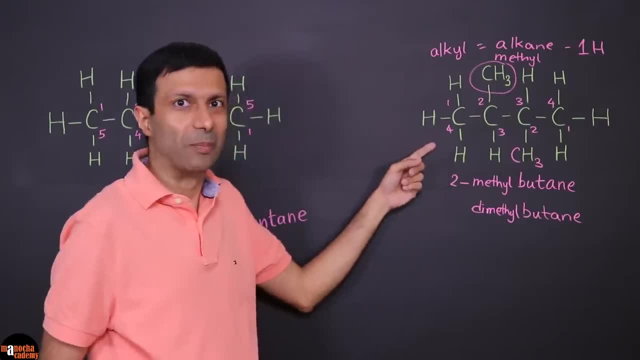 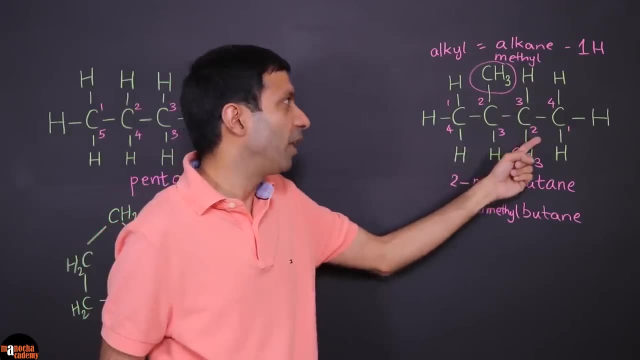 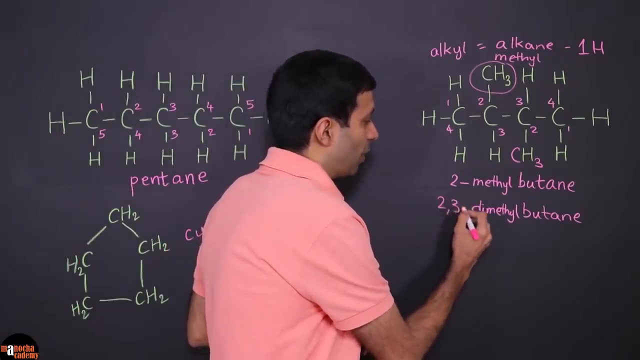 either i have to go with the top, the forward numbering, or the backward numbering, so it's going to be 2 comma 3, or if you use the backward numbering, it will be 2 comma 3.. so both the numbers are same. we chose. we have to choose the smallest number, so it's same anyways. so we are. 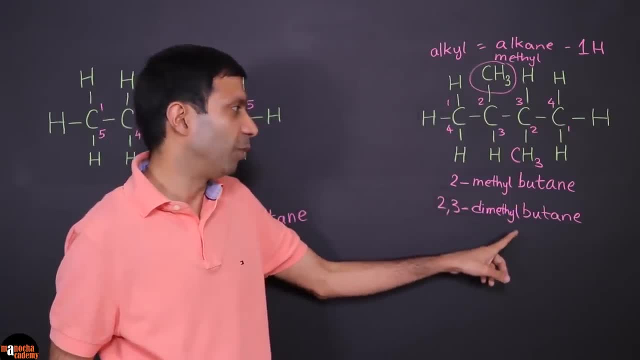 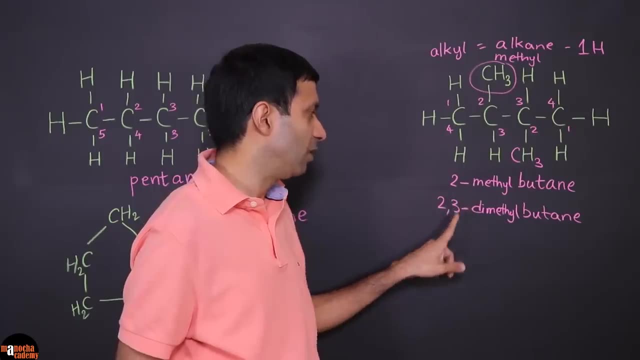 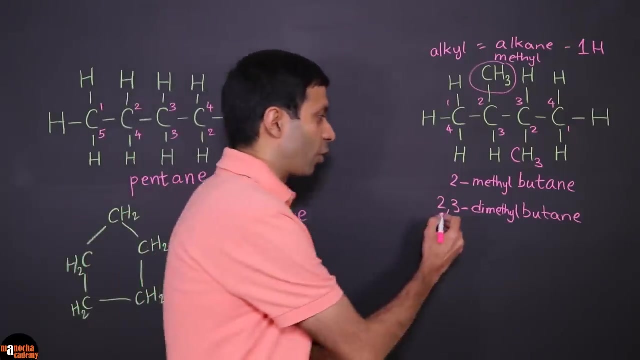 going to write. it's 2 comma 3 dimethyl butane. now note some important points here. between the number and the letter there's always a dash, as you can see here or here. so between the number and a letter, and if you have two numbers, like here, there's a comma in. 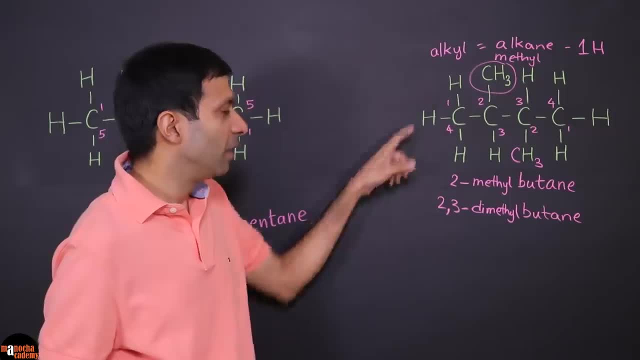 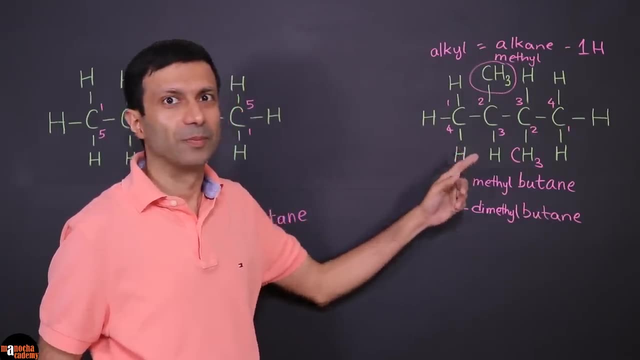 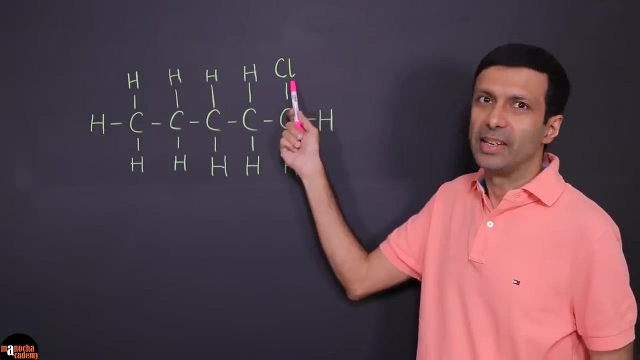 there. can you see the comma? so this one would be 2 comma 3 dimethyl butane. that's the iupac name of this compound. now let's take a look at this compound. so what's interesting here is that there is a chlorine in here. but again, first ignore the chlorine and look at the longest continuous. 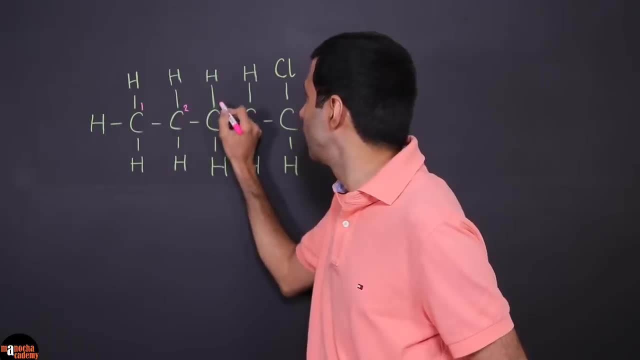 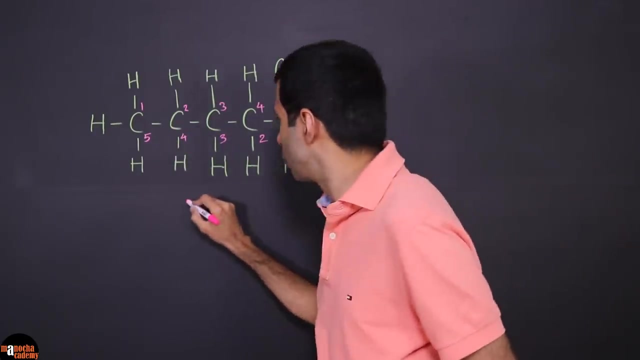 carbon chain. so let's go ahead and number it forward and backward. and we have one, two, three, four, five carbons, and i'm going to number it backwards also. so if we ignore chlorine, what is the basic name here? it's five carbon. so that's a pent and, as you can see, there are only single. 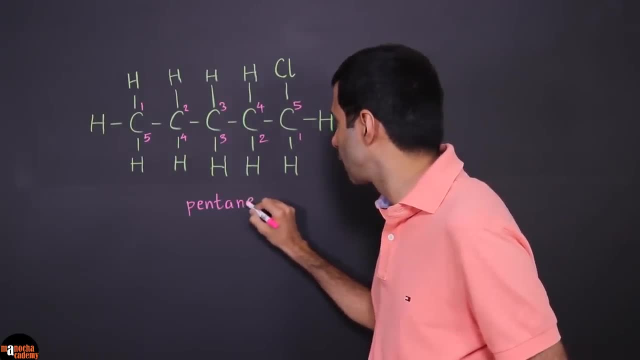 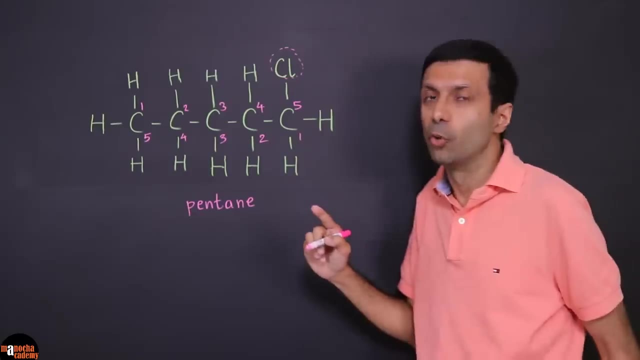 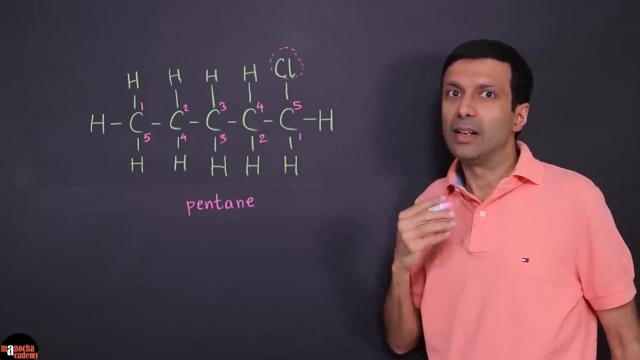 bonds here, so it's a pentane. now this chlorine is a halogen and so that's our functional group here. so we have the halogen functional group and remember for halogens and for the alkyls that we had done, the name goes in the prefix. 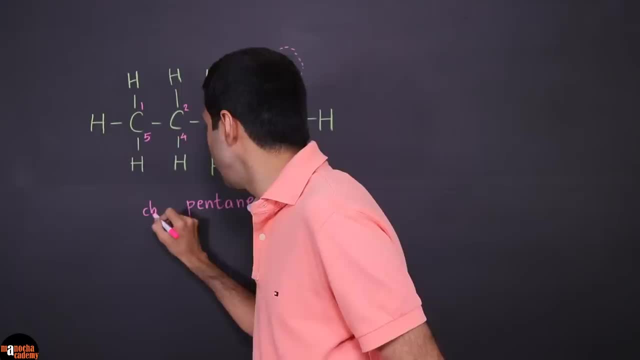 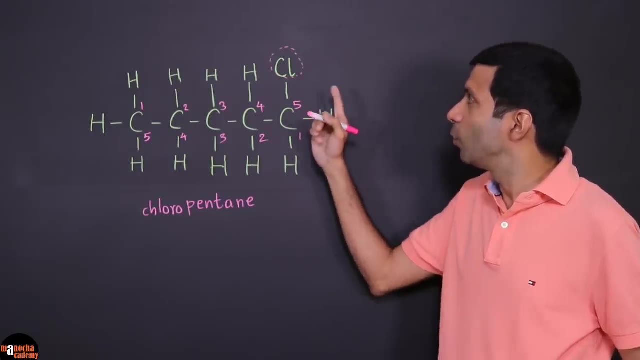 so it's going to be a chloropentane, not chlorine pentane. it's chloropentane. so that's the way iupac, iupac name is done and we also need to give the position. so what position of chloro should i give? 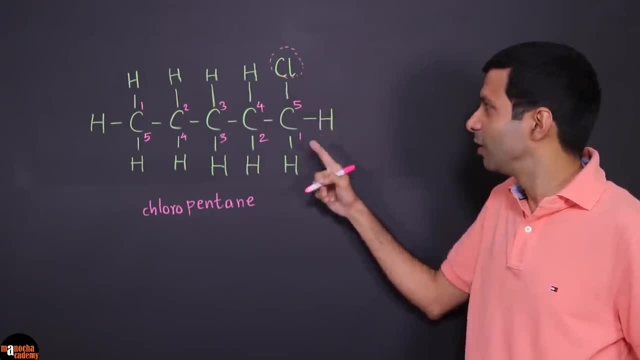 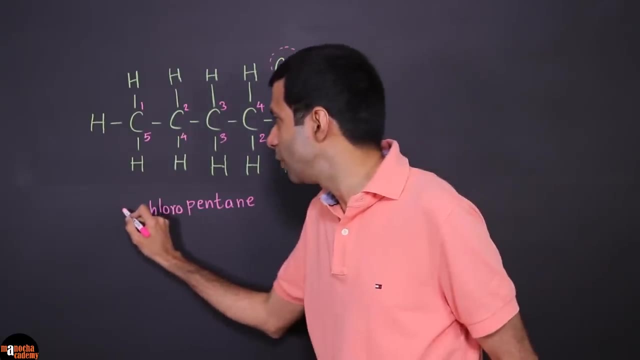 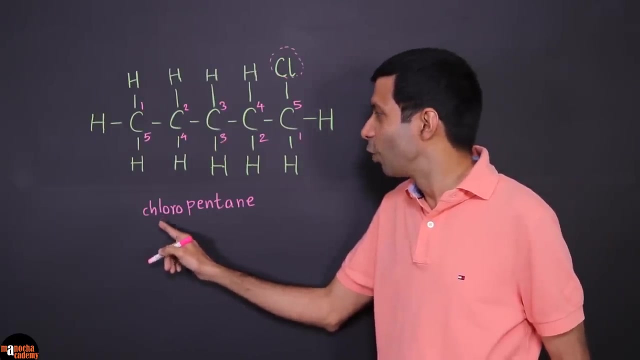 here, is it going to be five chloro? no, it's one chloro, because we'll choose the nearest number, the smallest number here. but there's no need to actually write one chloro here, because the number one is not necessary. so simply, the name is going to be chloropentane. but if the 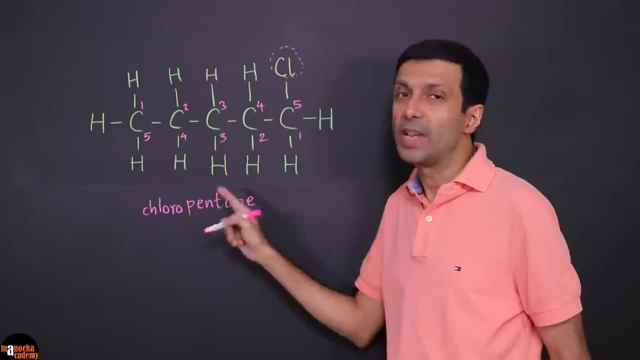 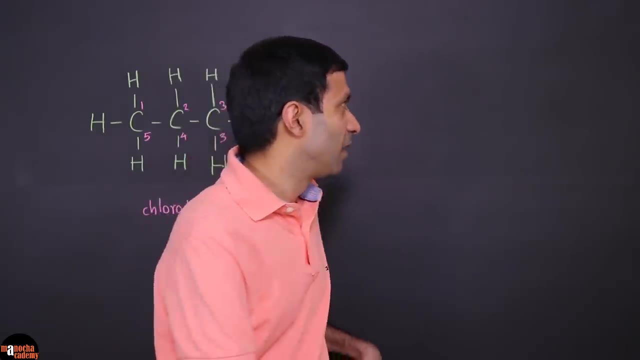 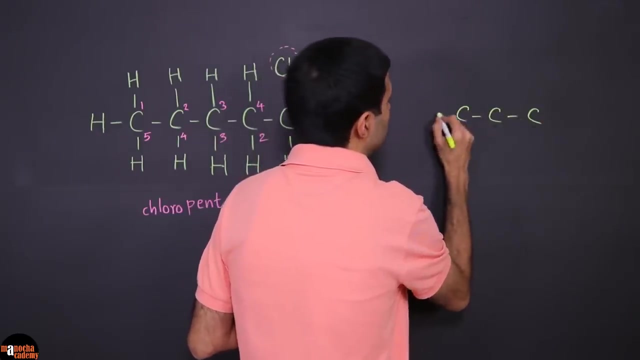 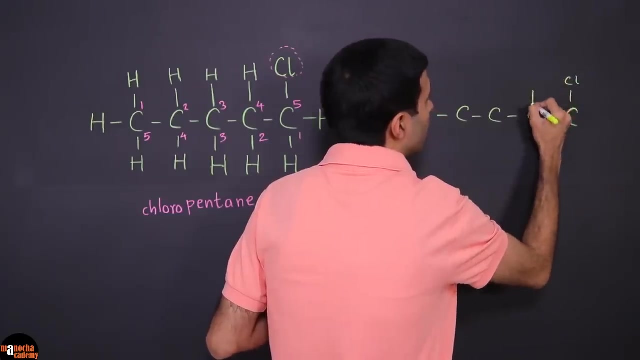 chlorine was here, then the name would have been 2- chloropentane. right now, let's take a look at another example. so let's say again: we have five carbons here and we have a chlorine in here, a chlorine in here and, let's say, bromine in here. 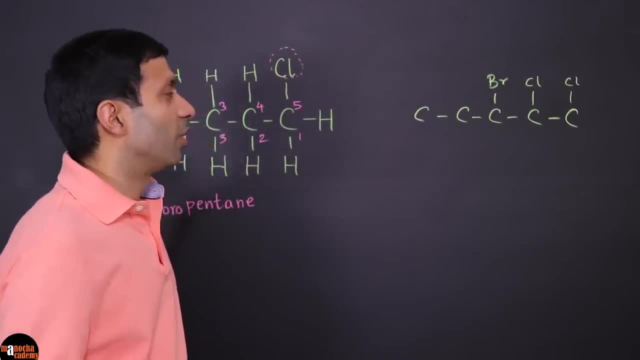 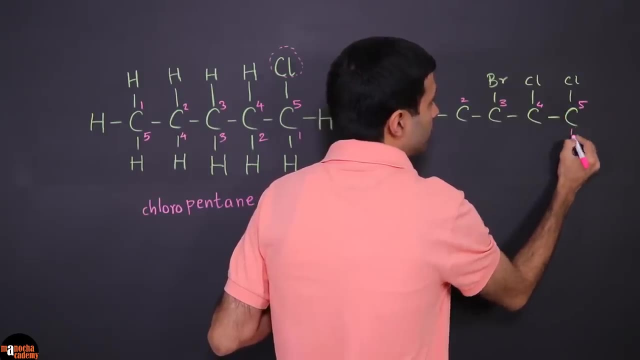 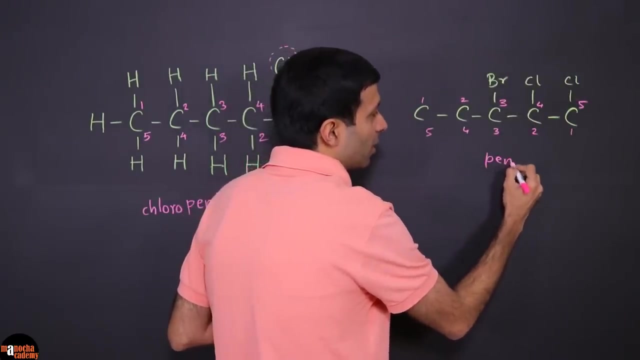 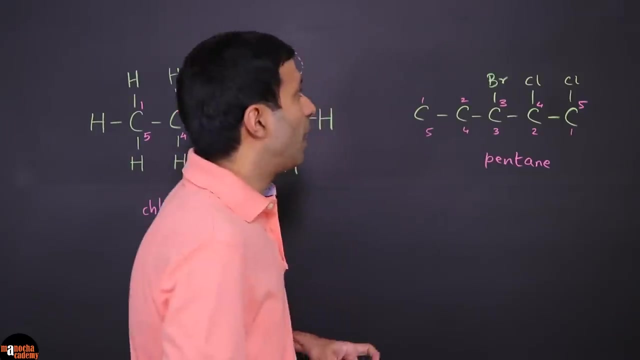 i'm not drawing all the other hydrogens. so again we'll number our carbon chain forward and backwards, so it's five carbon. we'll ignore this for a moment, so that's the simple way to do it. so you'll have a pent and only single bonds, pentane. now again, we have some halogens in here, so there are two chloro. 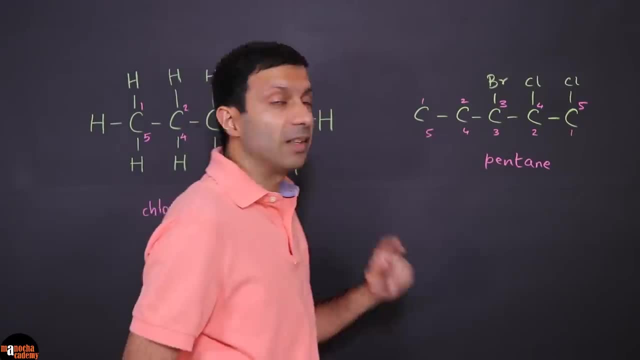 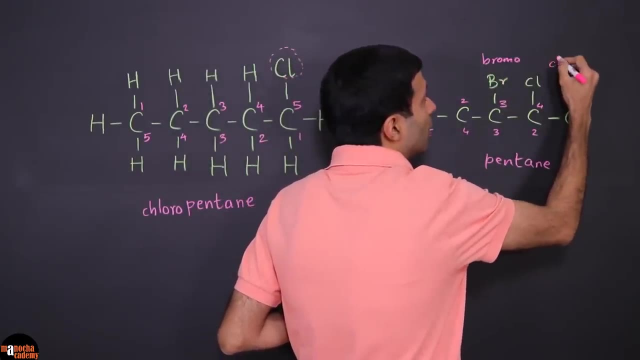 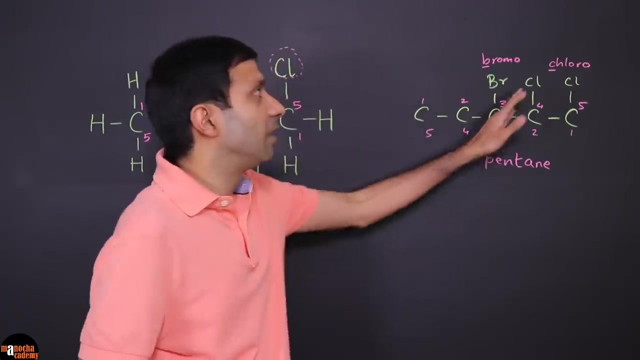 and a bromo right now. there's another rule that comes in here: when you have a bromo and and a chloro, you need to go in alphabetically. you need to go in alphabetically. you need to go in alphabetically order. so b comes before c. you shouldn't consider the dichloro, the d is not important, we are 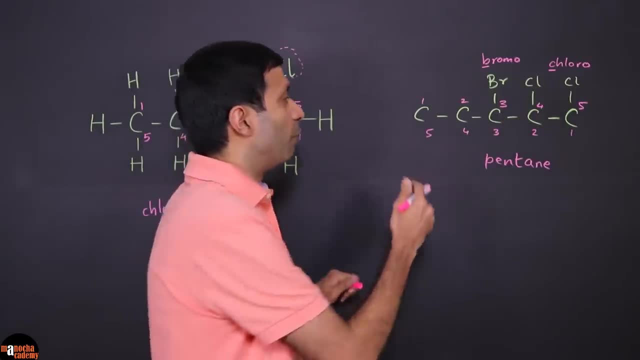 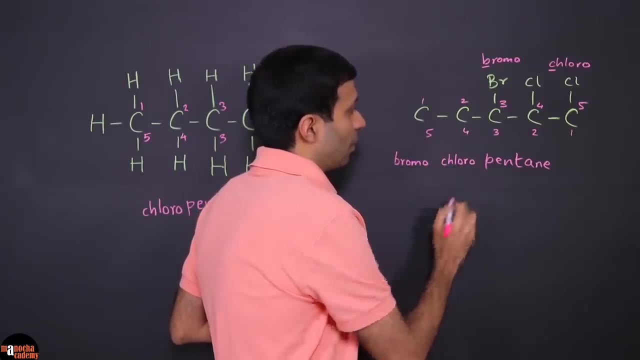 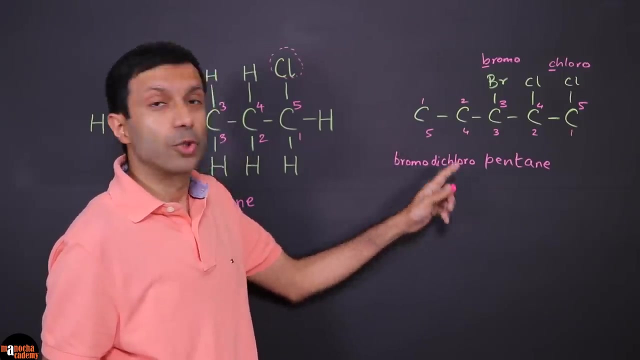 comparing bromo and chloro, so the name bromo will come here first. so there's a bromo and there's a chloro, sorry, dichloro. right, so there's a bromo and dichloro, but we also need to give the numbering and remember we need to choose the smaller numbers. 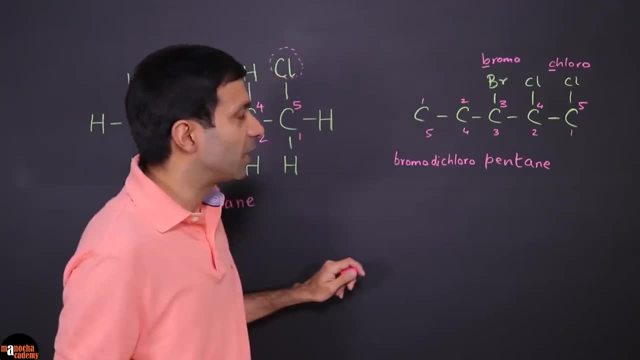 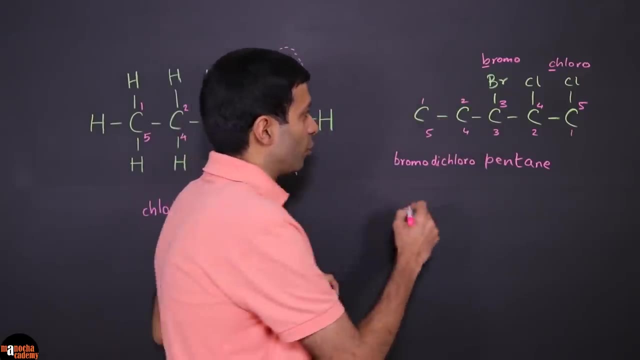 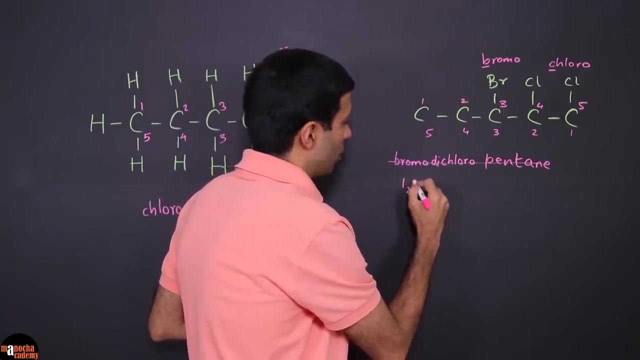 so we won't go for this scheme. we'll go for the backwards scheme. you can see that there's a 1, 2 dichloro and a 3 bromo, so i'm going to rewrite this name again as so let's cancel this out. it's going to be 1 comma. oh sorry, it's going to be three bromo. 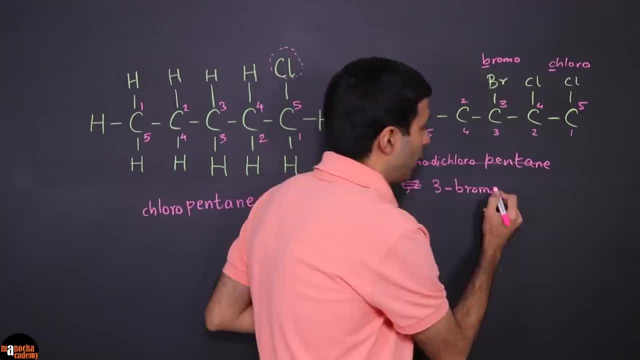 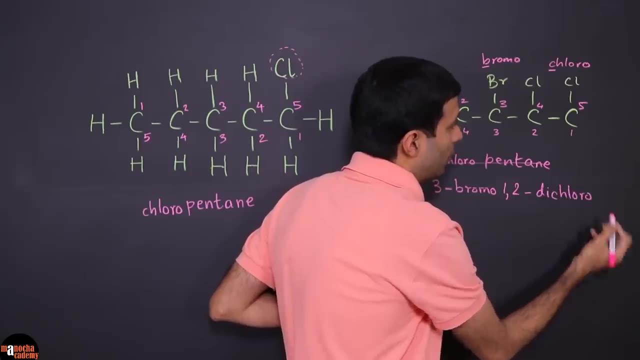 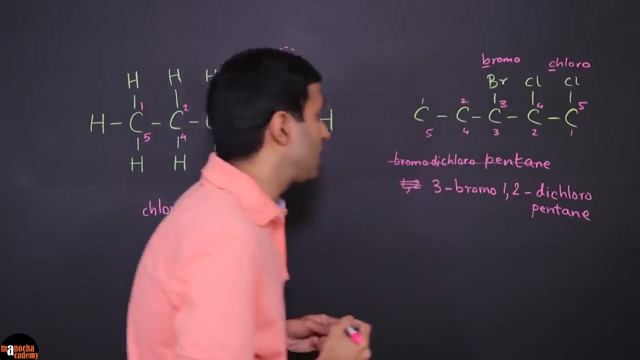 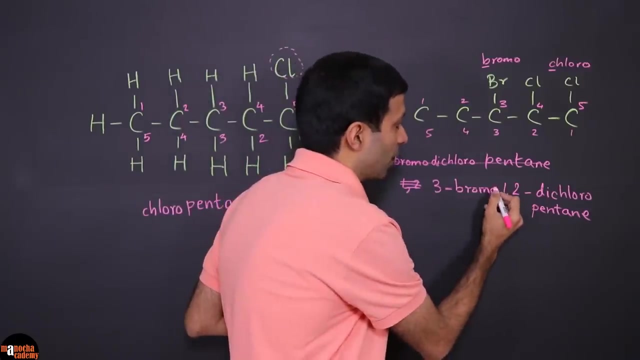 right. so the bromo is at position number three and after that we have 1 comma, 2, dichloro, correct and pentane. So note these things carefully, that between the number and the letter you can see there's a dash, between the numbers there's comma and there's a number and a letter here. so again a dash and we went in alphabetical. 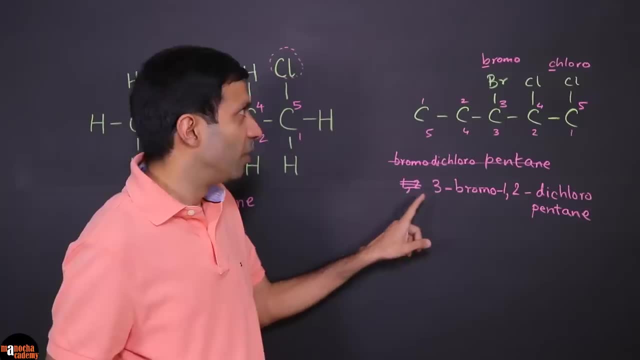 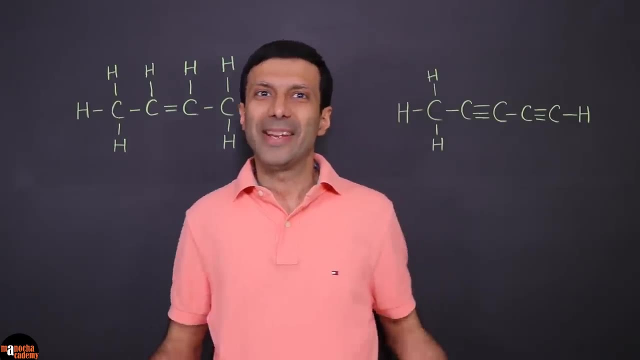 order. bromo b came before chloro, So you can see it's a: 3 bromo, 1 comma 2 dichloro pentane. All right, let's try the next one here. So what's the name going to be? Again, let's. 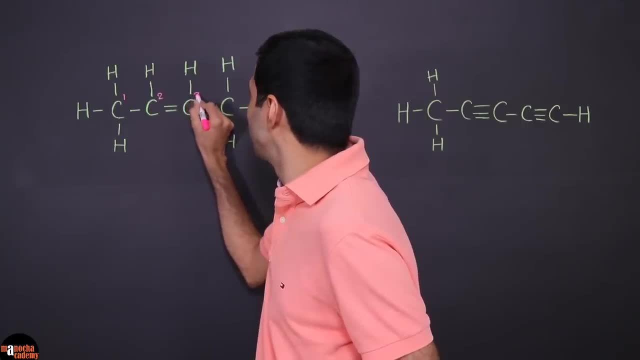 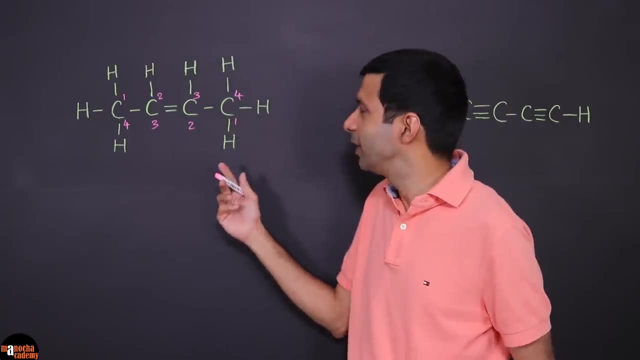 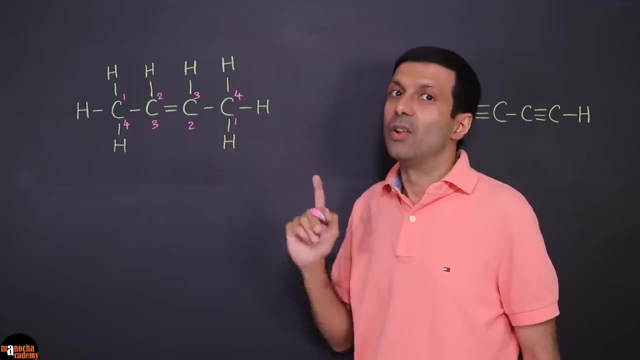 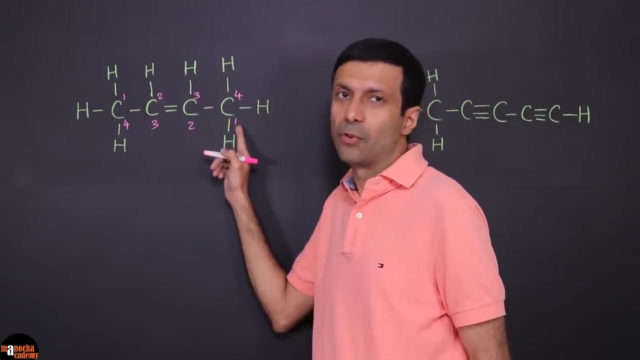 number the longest continuous carbon chain. So we have four carbons here. so the name will definitely have butane in it and there's a double bond. So is this compound's name going to be butene? No, because the double bond is not at the first position or over here, if you counted the 1 from here. 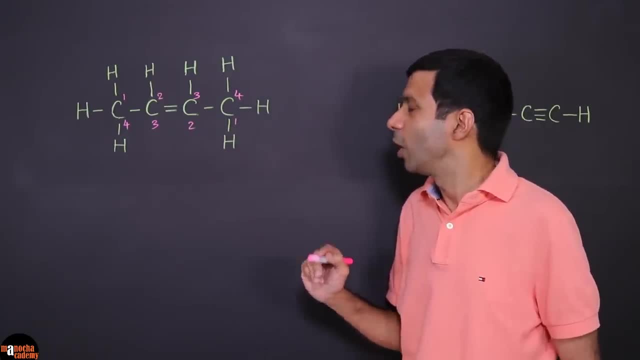 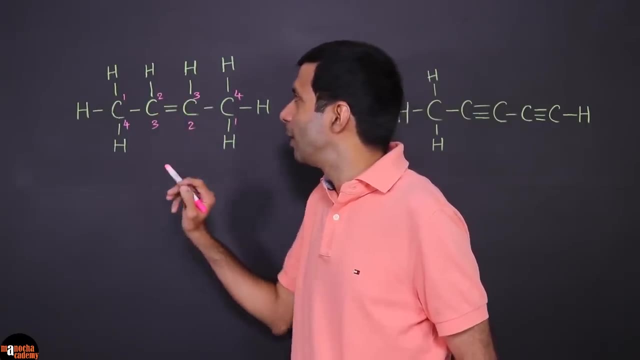 So we also need to give the position of the double bond. So how do we do that? The double bond is between 2 and 3. So we will choose the smaller number and say the double bond is at position 2.. 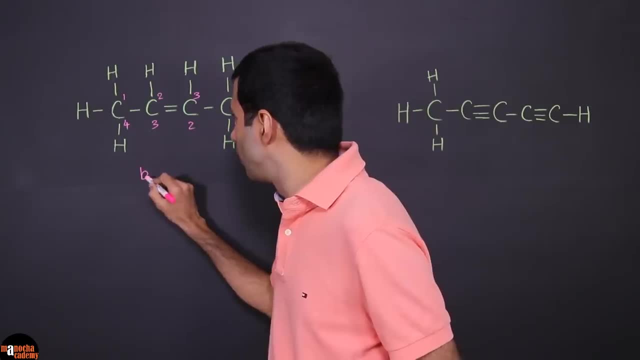 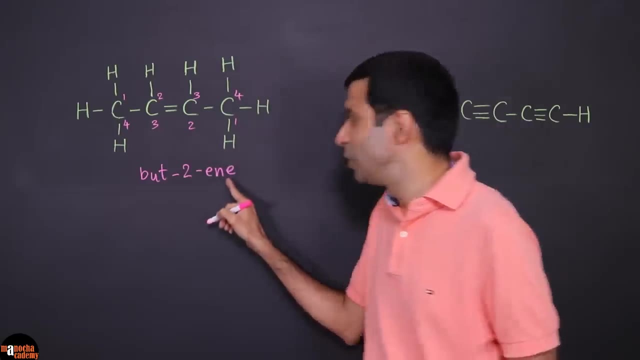 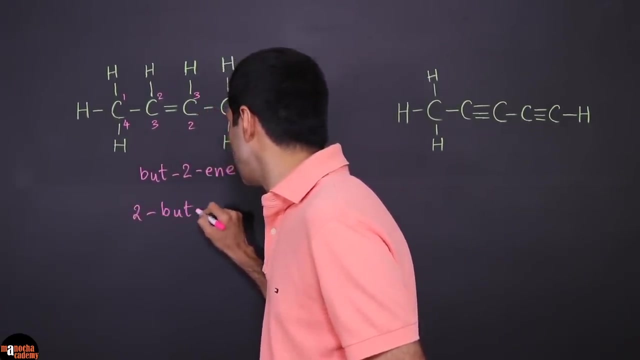 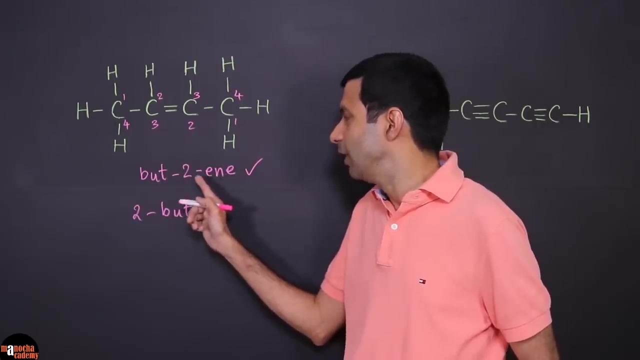 So the name is going to be butene, because we are giving the position of the double bond. Sometimes you may see this compound written as 2-butene also, But usually this is the recommended style where we give the number in the middle here. 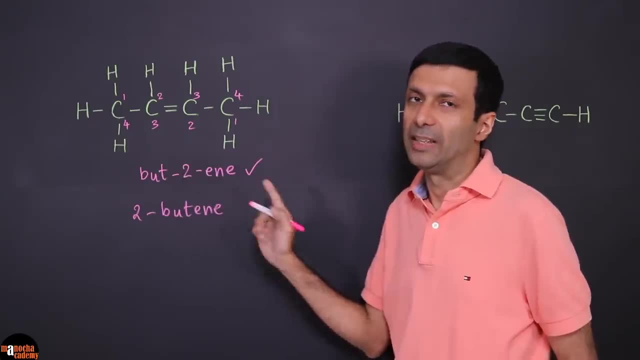 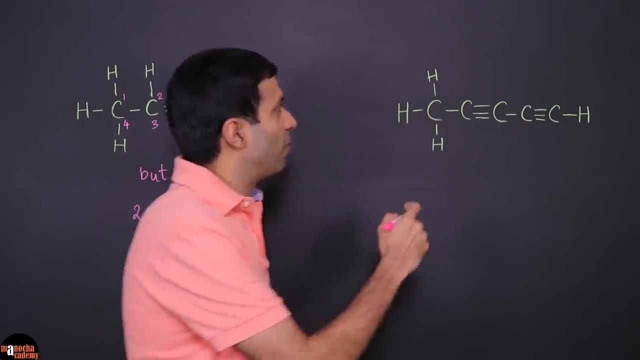 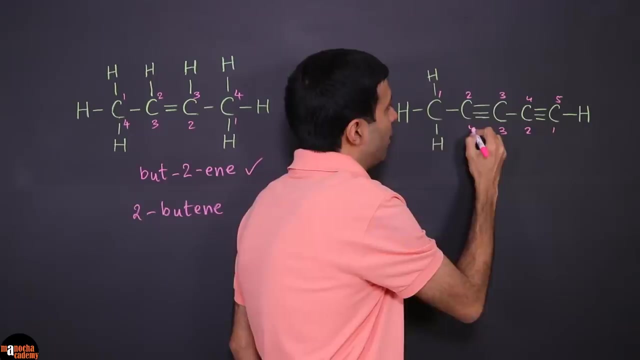 So it's 2-ene but-2-ene. Okay, now let's try this compound. So here, what do we have? We have a 5-carbon chain And there are some interesting triple bonds here, So you can see that there are 2 triple bonds. 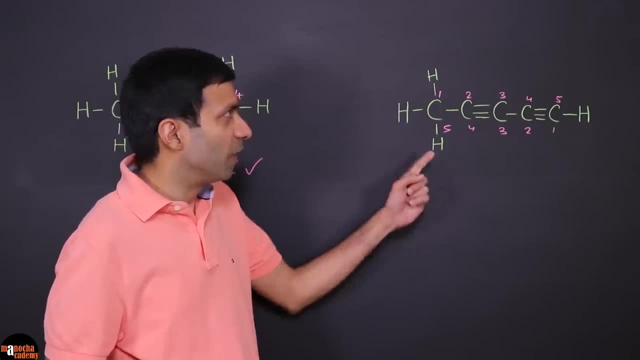 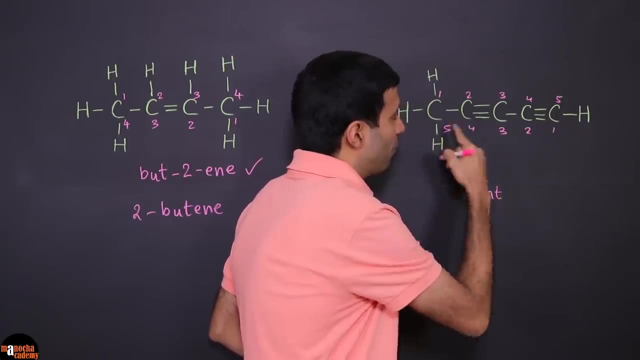 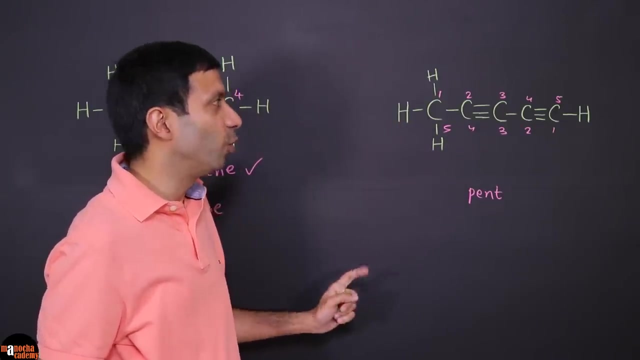 So is this going to be a pentine? No, because there are 2 bonds. So first the name is going to start with pent Because there are 5.. So there are 5 carbon atoms here And it's a di-ine because there are 2 triple bonds. 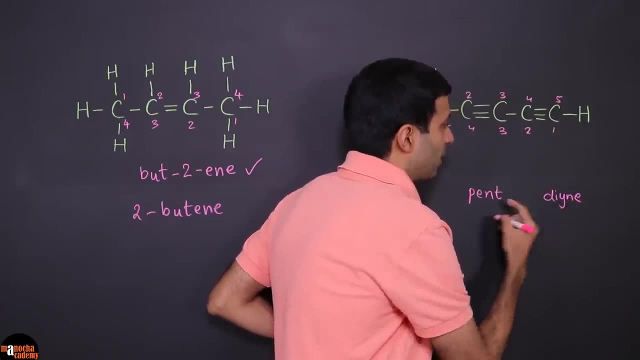 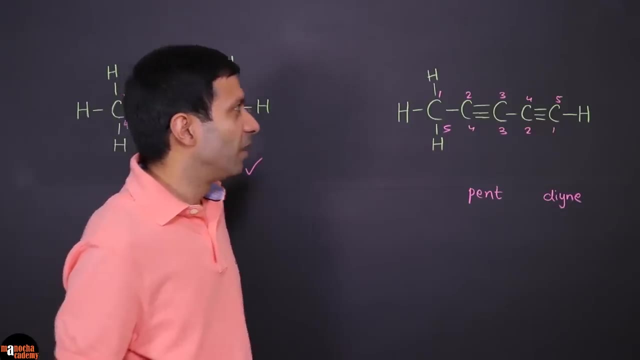 So I'm going to write that here. It's a pent-di-ine, But I need to specify the position of the triple bonds. So what's the position going to be? We can say the triple bond is between 2 and 3 and 4 and 5.. 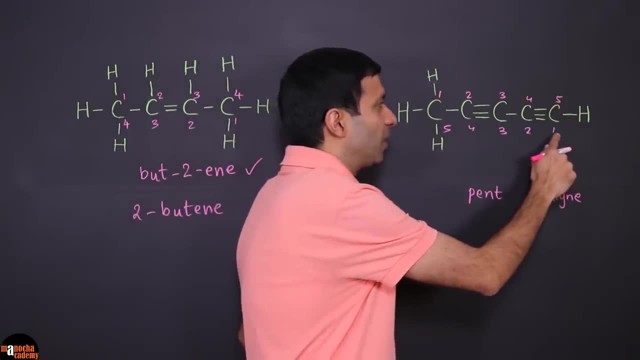 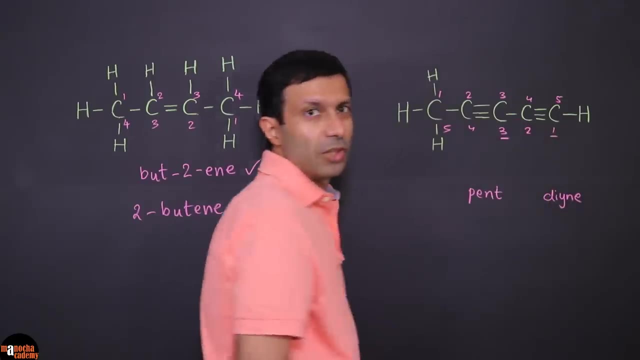 But that's using the bigger numbers, So let's go for the smaller numbers. So we'll start counting from here. So the triple bond It's between 1 and 2 and 3 and 4.. So we'll use these position numbers. 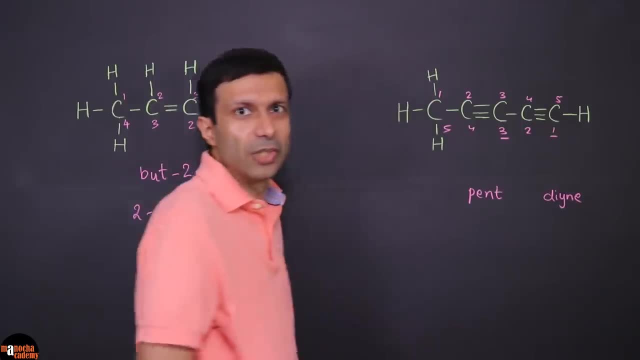 Because we are saying the triple bond is at position 1 and position 3.. So the name is going to be pent-1,3-di-ine, And again, between the letter and the number there's a dash, And between 2 numbers there's a comma in here. 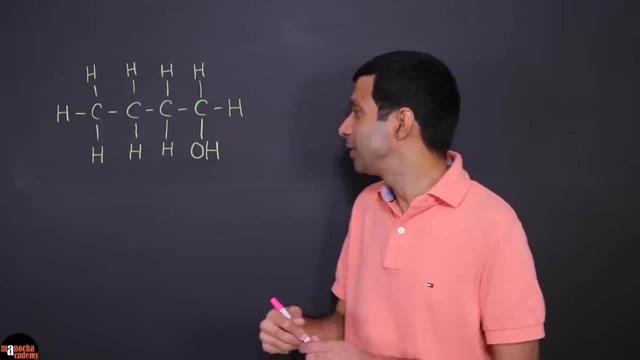 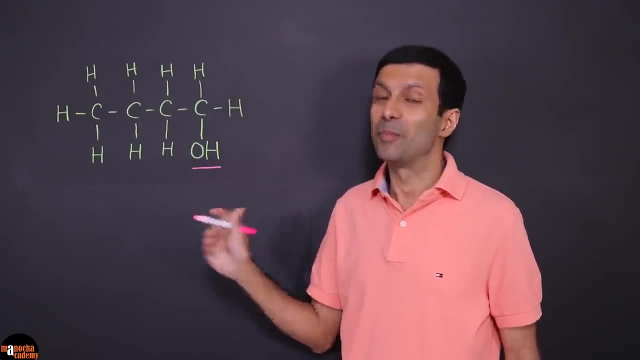 Alright, let's name this guy now. Now, what's interesting here is there's the OH functional group. So this is an alcohol, But again, to simplify things, we are going to ignore OH and look at the longest carbon chain here. 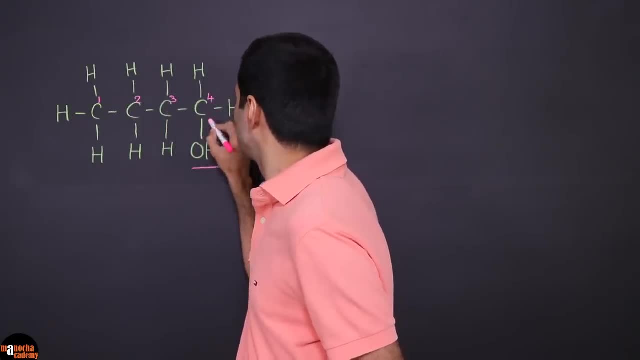 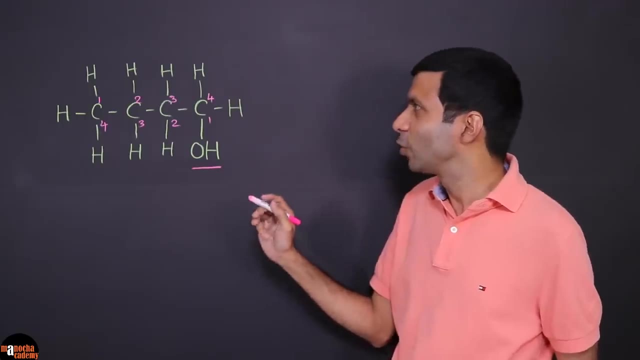 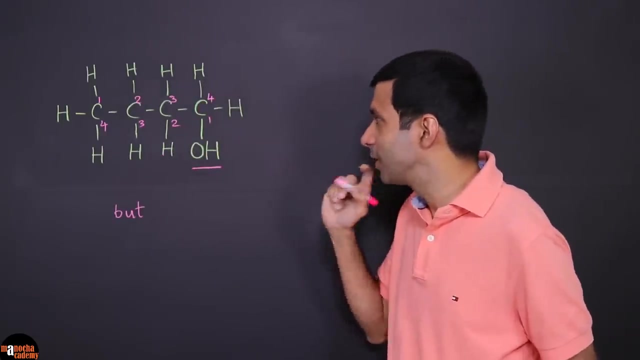 So let's number it here Forward and backwards, So there are 4 carbons. So basically, the name is going to be a butte. It's going to start with butte, And if the alcohol wasn't there, the name would have been butane. 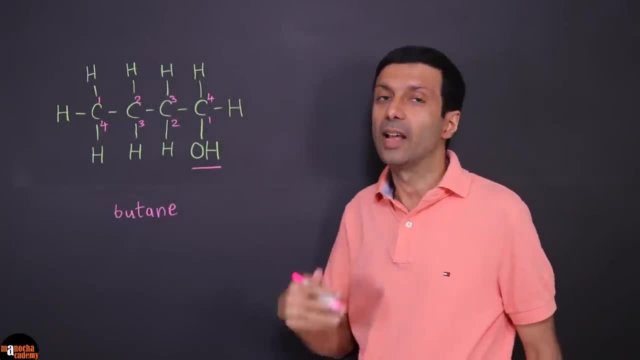 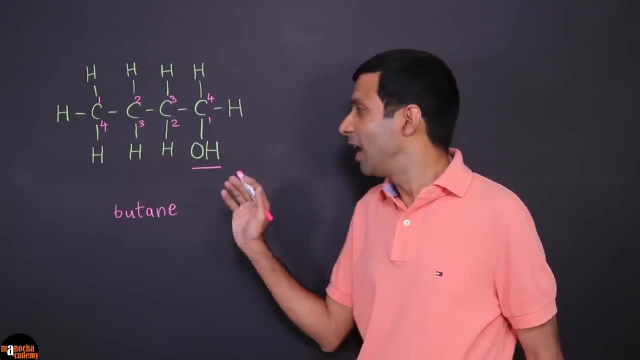 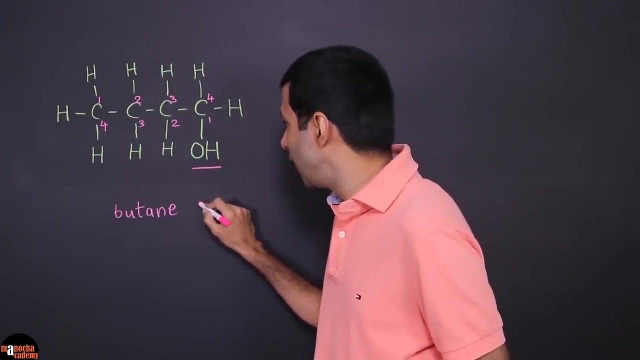 But you know that alcohol and other functional groups that we are going to talk about, their name comes in the suffix. The prefix was for alkyls and the halogens. So this alcohol name will come in the suffix and the name ends with OL. 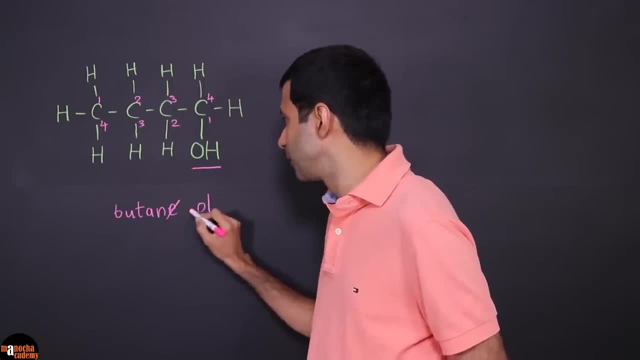 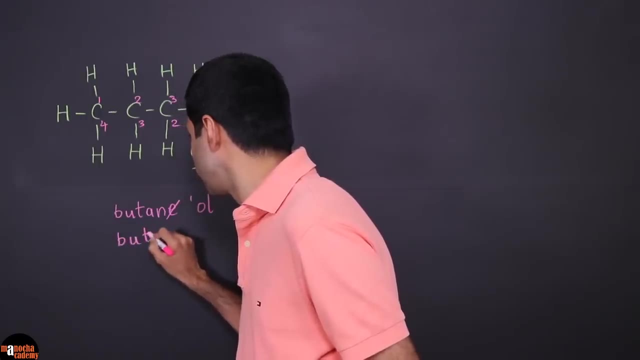 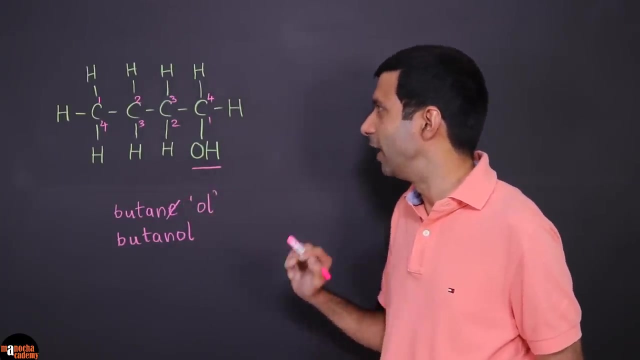 Now, when you add OL, you need to remove the E, So this OL gets added to the name and the name basically becomes butanol. So remember, the E is removed and we attach the suffix OL. And what is the position of butanol? 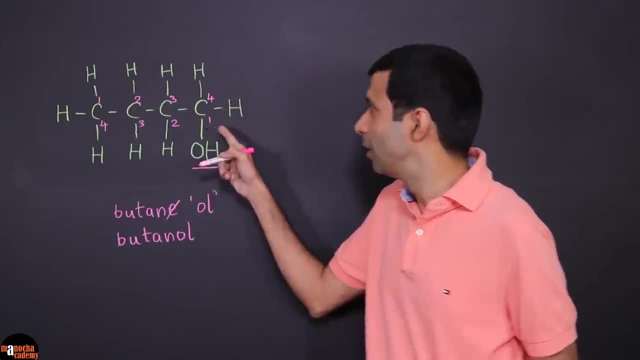 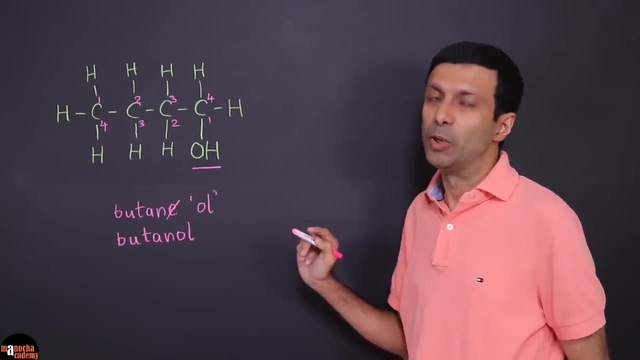 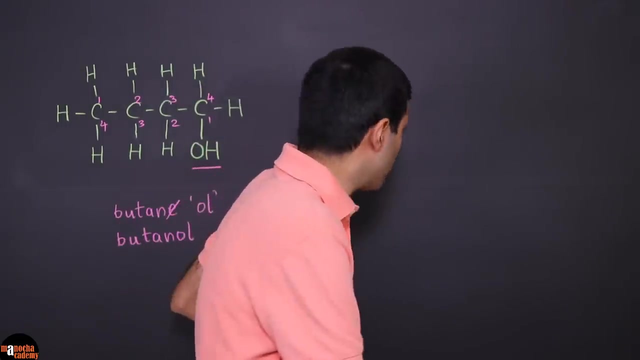 It's at position 4, but we'll choose the number 1 here because that's the smallest number. So it's basically butan-1-ol or basically butanol, because we don't have to write the number 1.. Now let's say the OH was at a different position. 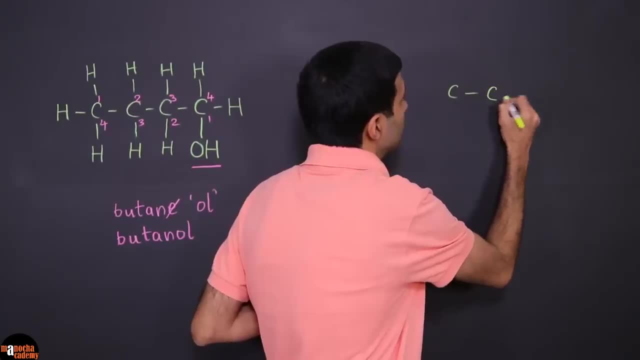 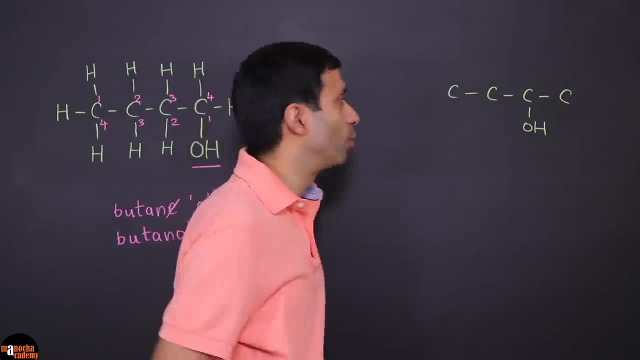 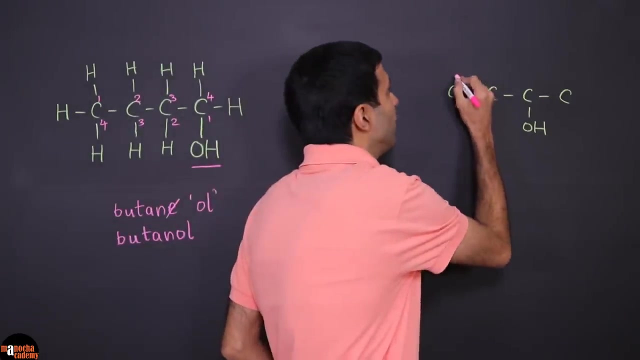 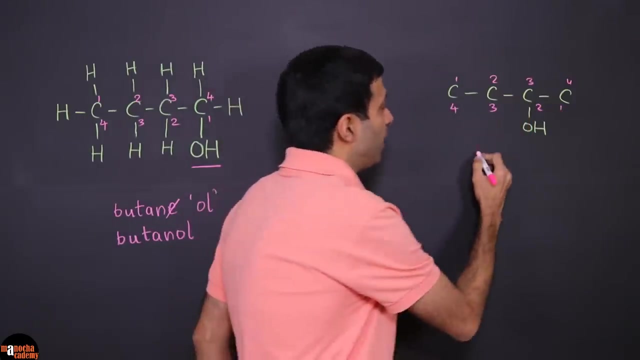 So let's say we had something like this, And the OH was here and rest, of course, are hydrogens. So what will be the name of this compound? Again, we'll number our longest carbon chain, So this will be bute. 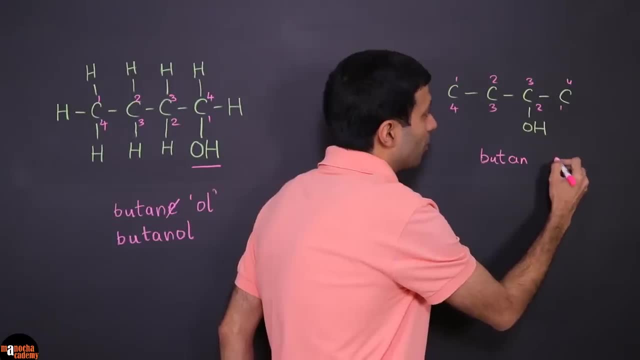 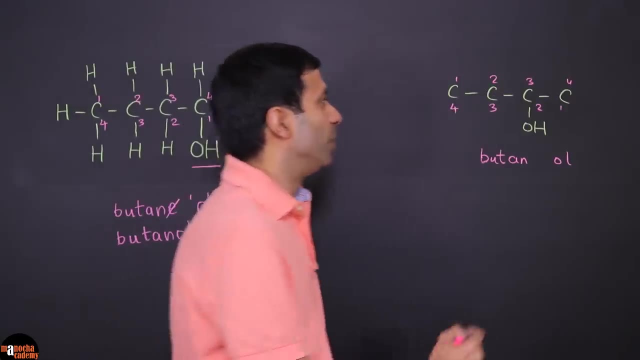 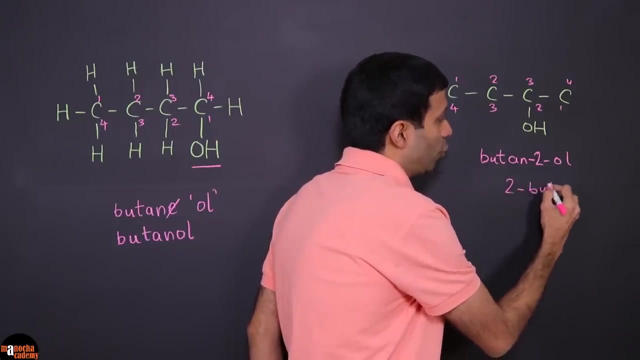 It will start with bute and the name would have been butanol, But the position of OH is on 2 because we'll not take 3, that's the larger number. So it's basically a butan-2-ol, or sometimes you might find it written as 2-butanol. 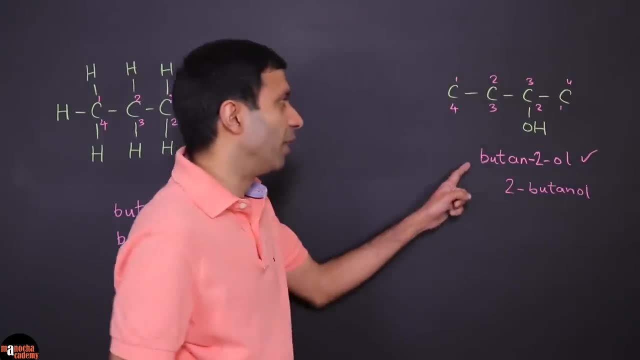 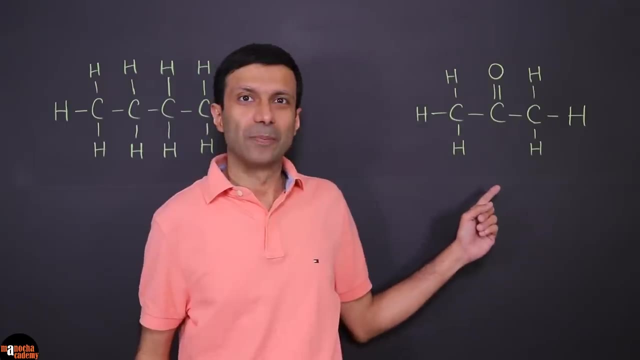 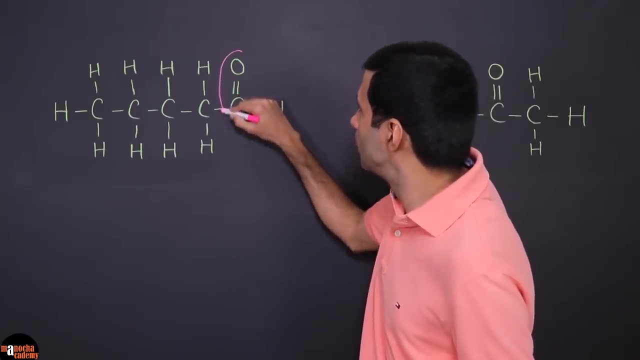 But usually this is the preferred way of numbering it: butan-2-ol. Now let's try to name these two compounds. Earlier we had seen the alcohol functional group. Here also there's a functional group. So do you know the name of this functional group which has C, double bond, O and H? 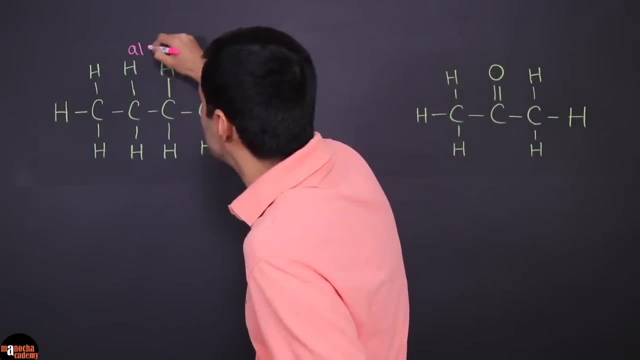 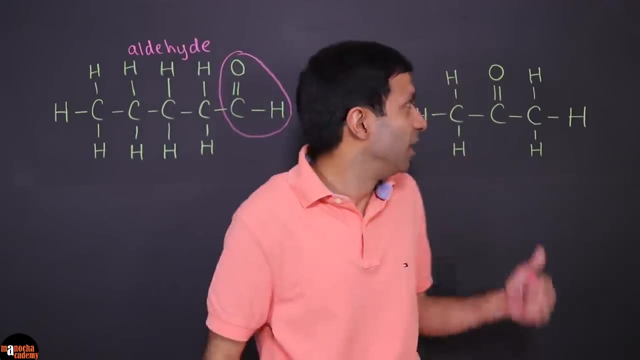 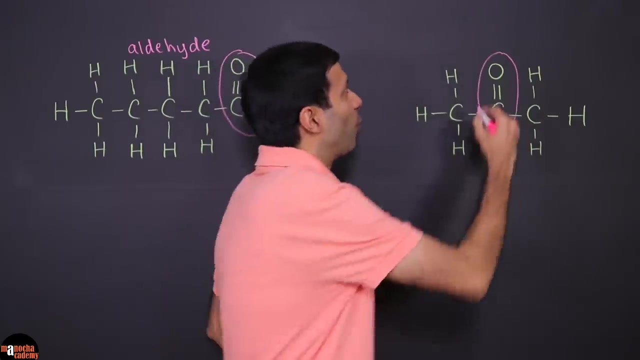 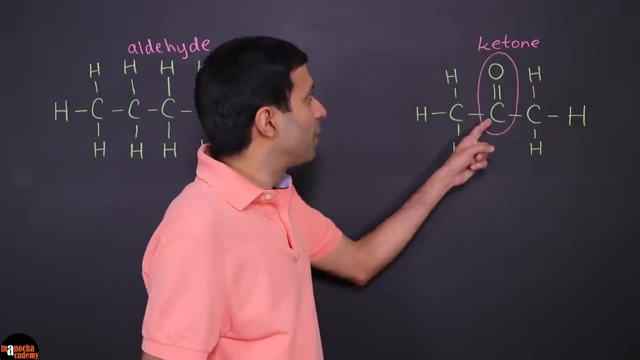 That's right. it's called aldehydes. And what is the functional group on this compound? This is our functional group and it's called ketone. So both the functional groups have C, double bond O on them. So what's the main difference here? 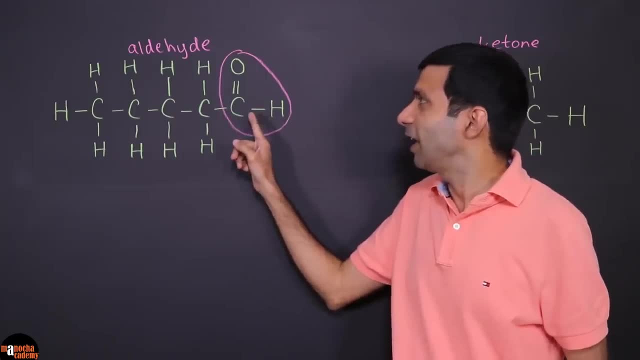 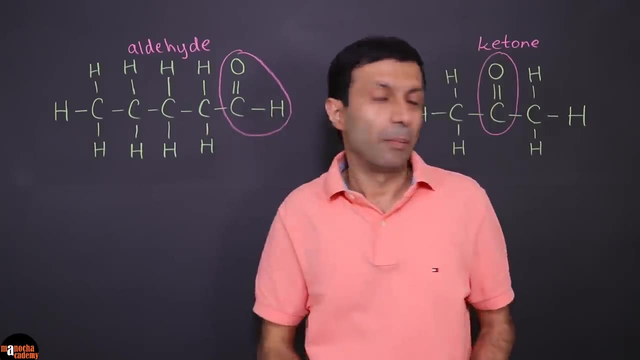 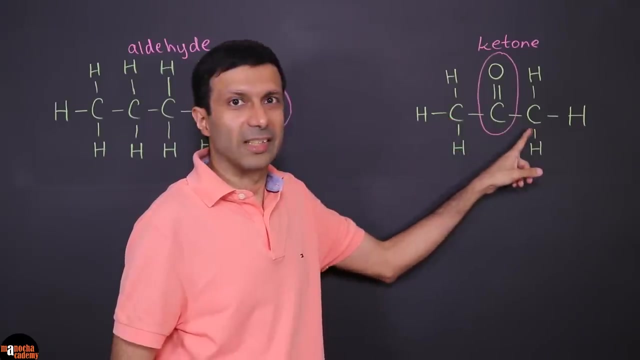 The aldehyde group is always at the end. So either on this carbon or it could have been here Okay, because it ends with an H. But the ketone group is interesting because the ketone group must have at least one carbon on both the sides. 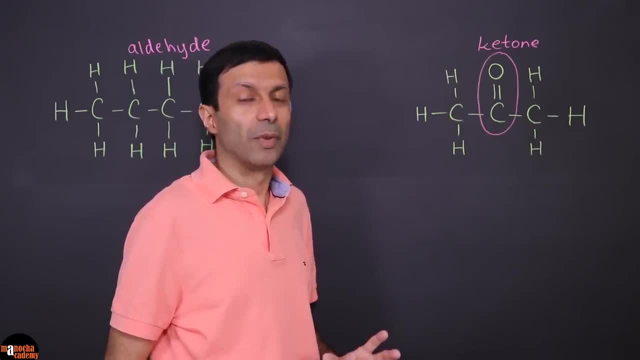 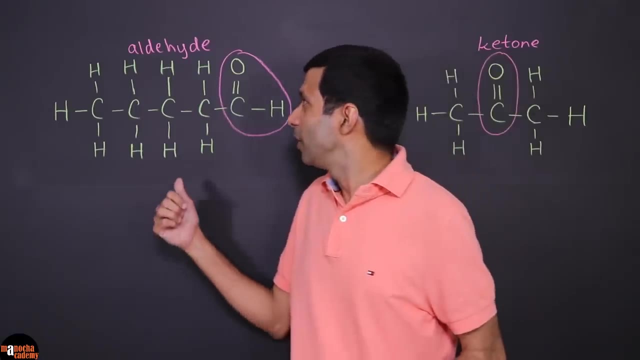 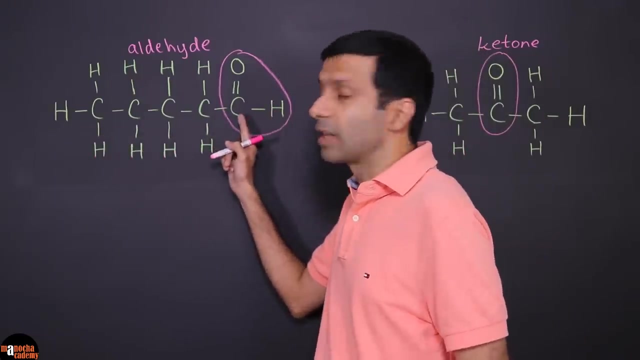 So that's an important difference to remember, Because the functional group decides the property of the compound and, of course, its name. So let's try to name this guy. So again, we'll apply the rule and look at the longest carbon chain. 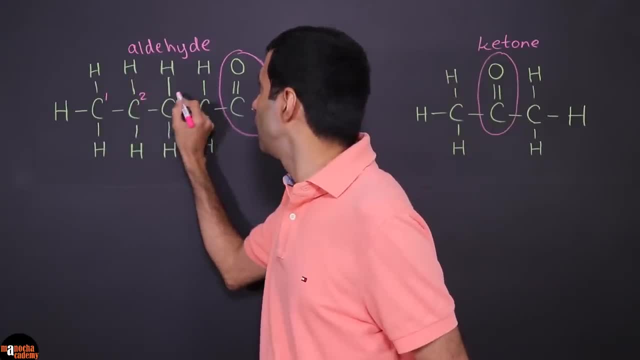 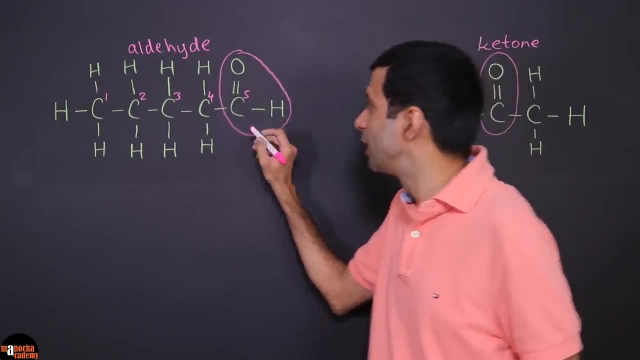 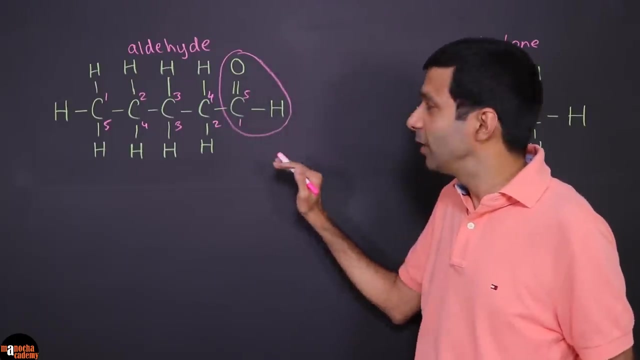 And one important point to remember is even the functional group carbon needs to be included in the counting. Okay, so it's five carbons including this one, And we'll also reverse number it. So if this functional group wasn't there, it would have been a pentane right. 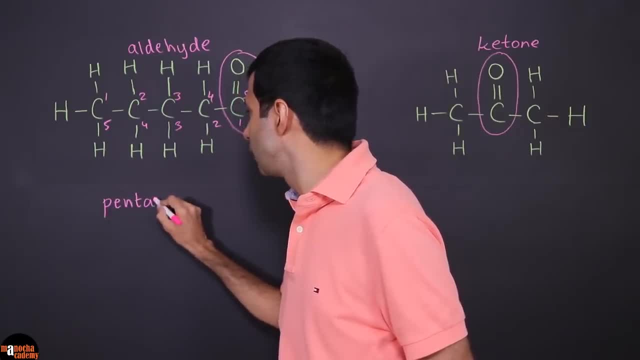 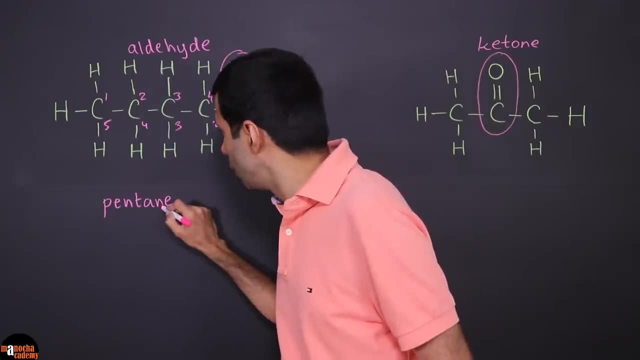 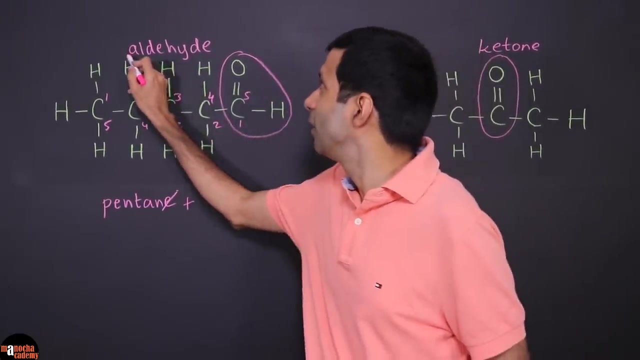 The compound would have been five carbon pent, and only single bonds are there if we ignore the functional group, So it would have been pentane. But the rule is to delete the E and add the suffix in the name for this functional group, And it's an aldehyde. 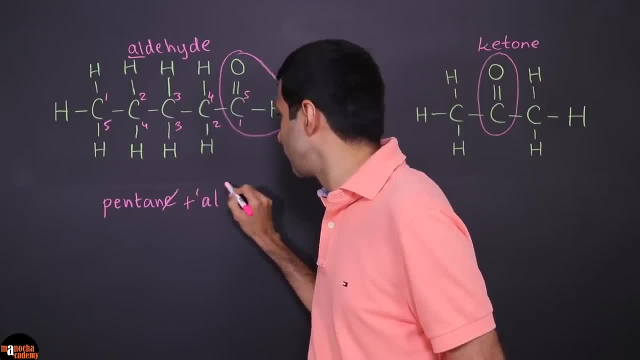 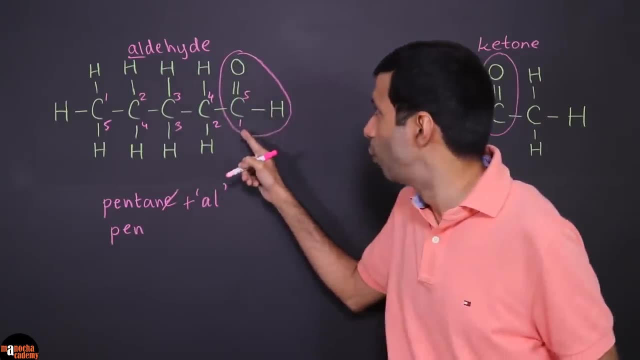 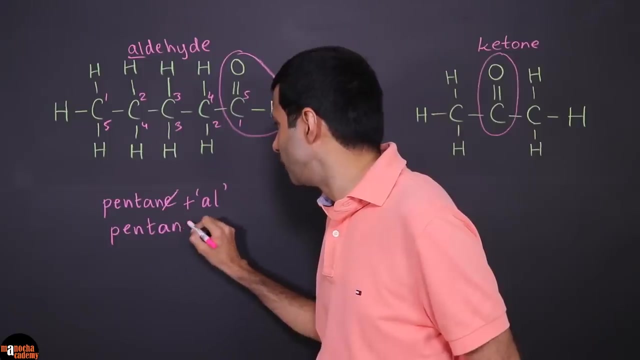 So we add the AL to it. So what will be the name of this compound? Pentanul, And it's at position one, the smallest number. So it's basically pentanul or simply pentanul. Okay, is that clear? 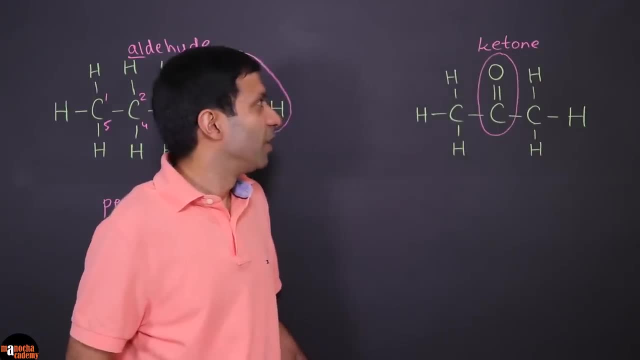 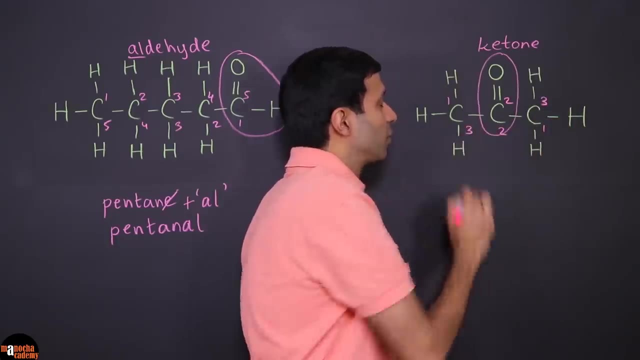 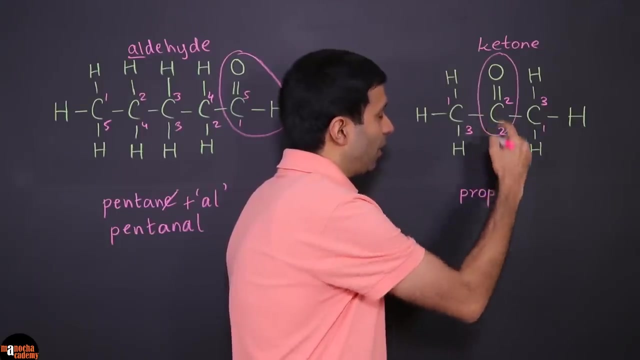 Now let's take a look at this compound. So here we have three carbons and we'll include the carbon of the functional group, So it's a three carbon chain. The name will be propane, right, If we ignore the functional group. 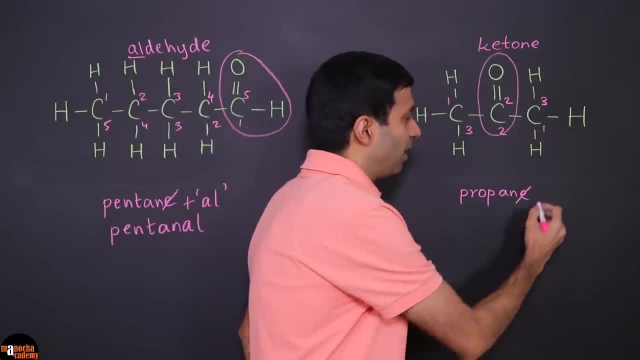 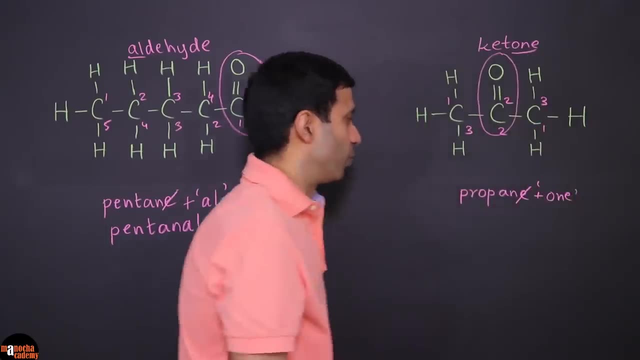 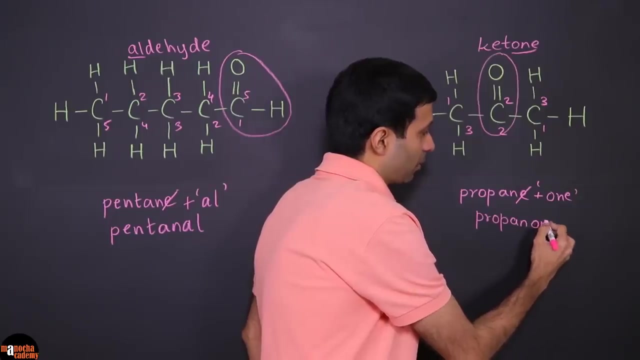 But again, the rule is we'll remove the letter E and add for the ketone we need to add on. So what's the name going to be? Propanone? Now you might be thinking we need to include the number also, right? 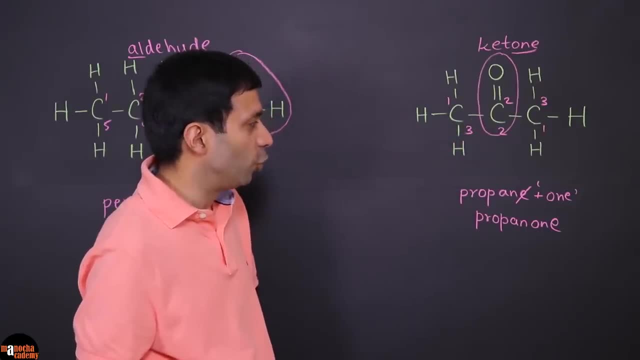 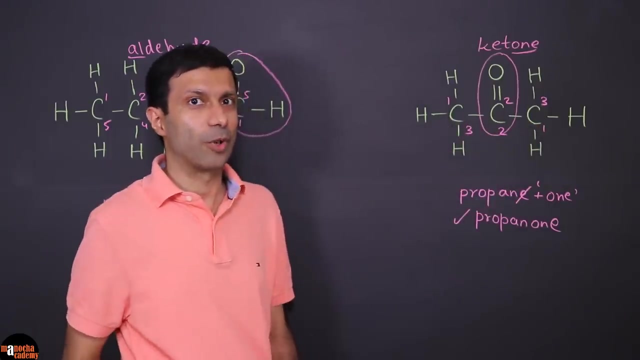 Because the functional group is at position two. So you might be thinking the name will be propanetone or 2-propanone, But no, the name is simply propanone. Why? Because 1-propanone or 3-propanone is not possible. 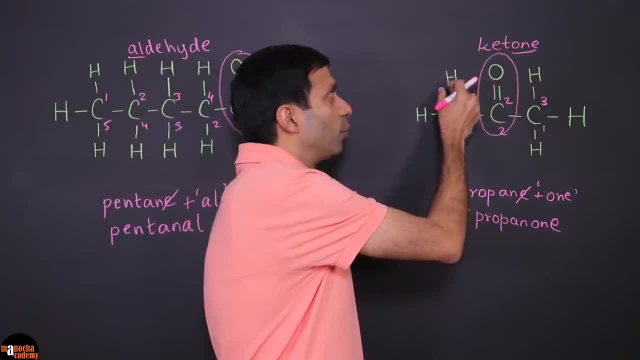 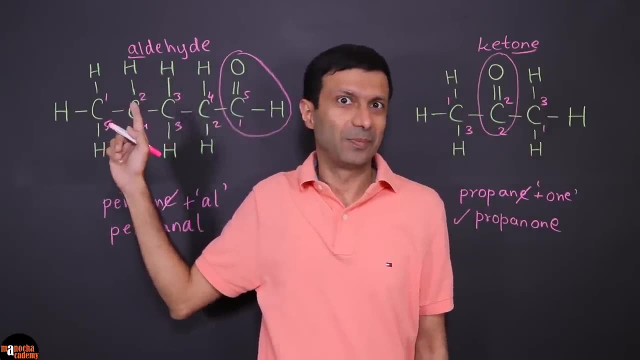 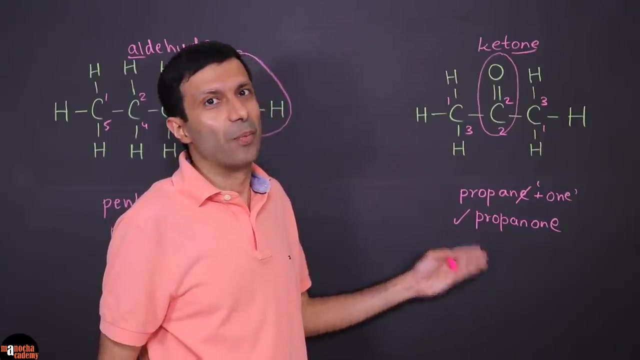 Because if I move this ketone group to this side or this side, if it becomes on the end, carbon, what will it become? It will be an aldehyde. So only possibility with three carbon is 2-propanone. So we simply write it as propanone. 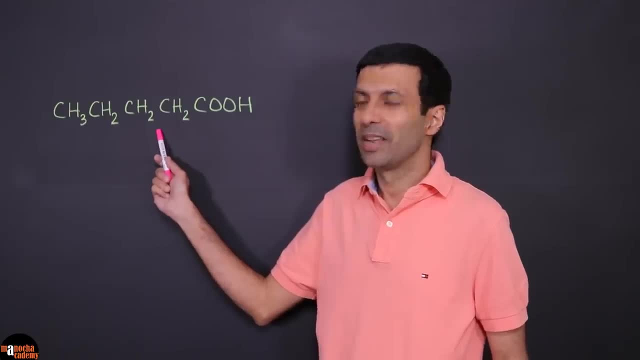 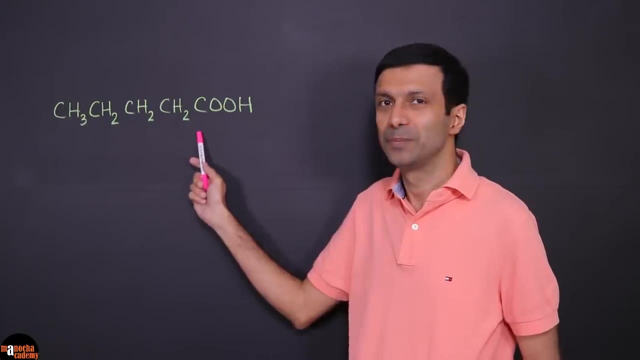 Now let's take a look at this example. I've written this in a condensed form because the whole structure with the hydrogens is not expanded here. Again, you should look for the functional group and can you see it? It's COOH. 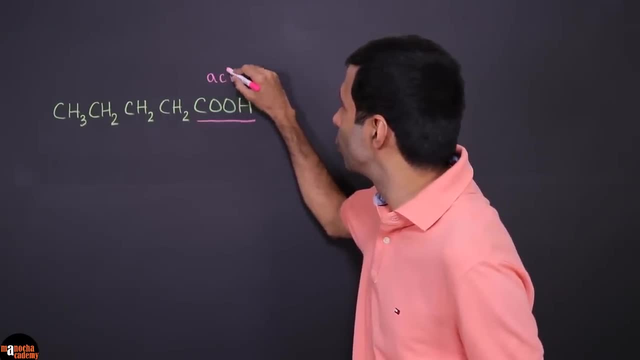 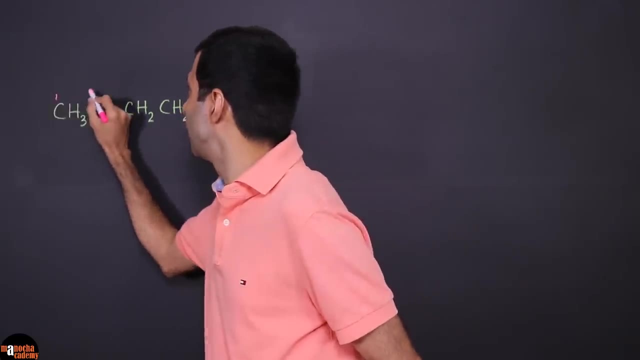 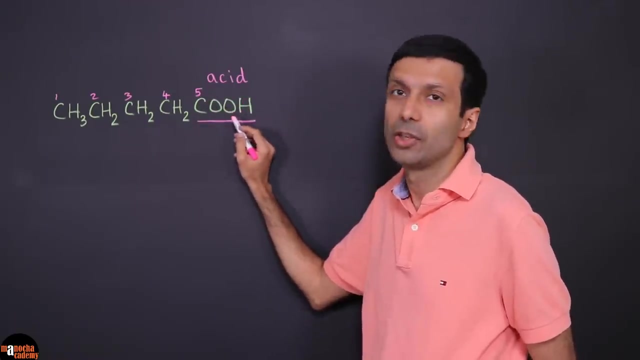 So this is a carboxylic acid. I'm just going to write simply Acid. here And again, let's count all the carbons in our longest carbon chain. So we have five carbons And remember we need to include the carbon in the functional group also. 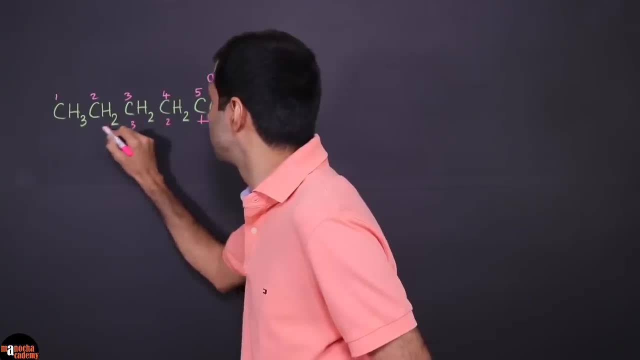 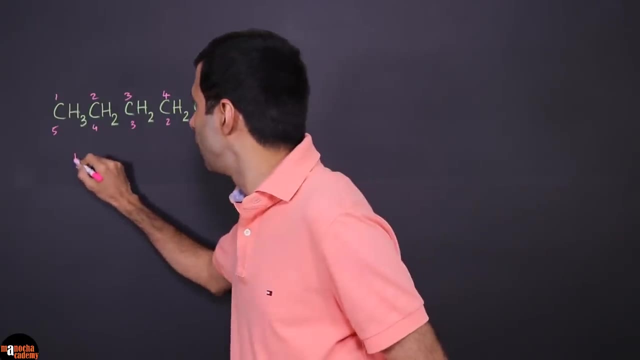 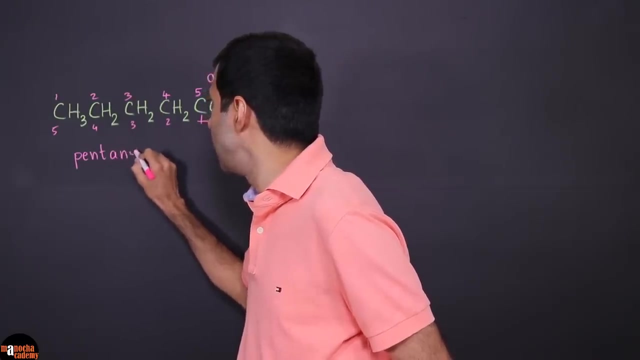 And let's reverse number it here. So if we ignore the functional group, the name would have been pent, because five carbons and all have single bonds between the carbons, So it would have been pentane. But this functional group's name will come in the suffix. And for acid the suffix is going to be oic acid. That gets added. So we are going to delete the E and add oic acid here. So what is the name of this compound? It's going to be pentanoic acid. 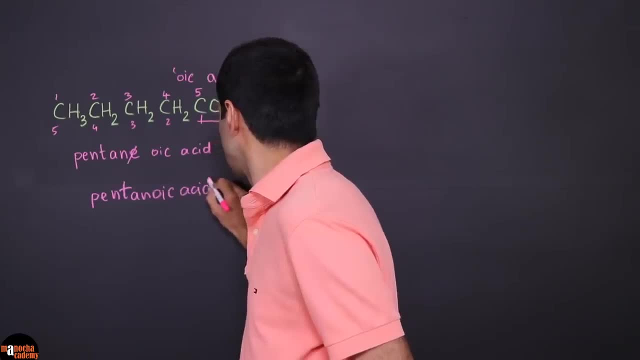 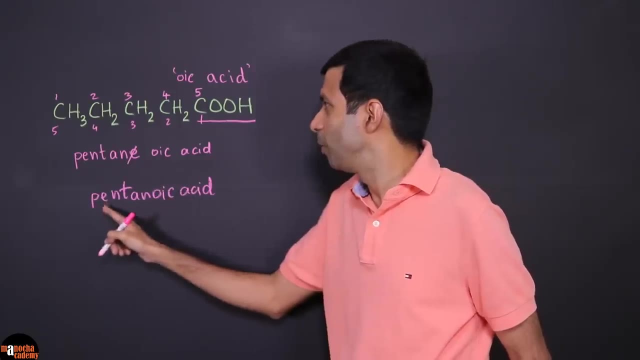 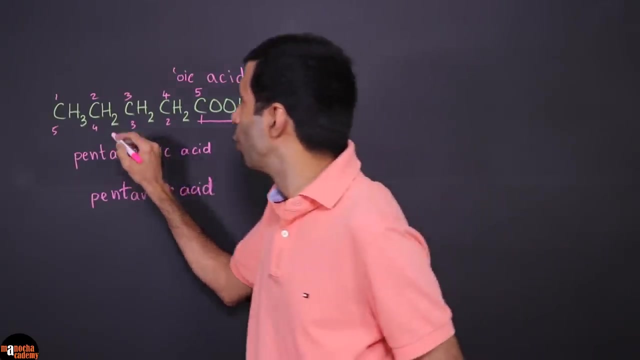 Right, And we don't have to give the position of this functional group because it's at position one. So it's pentanoic acid or simply pentanoic acid. Now let's say we have a chlorine over here, So I'm going to remove one edge and let's add a chlorine in here. 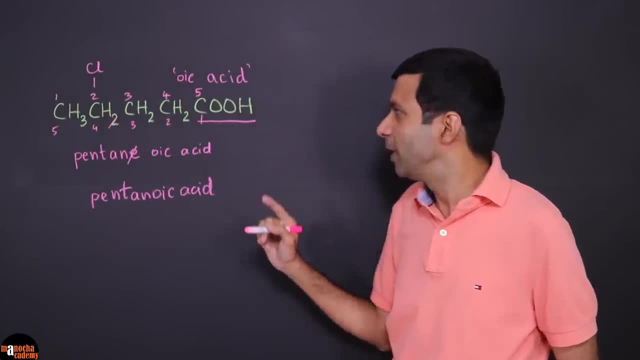 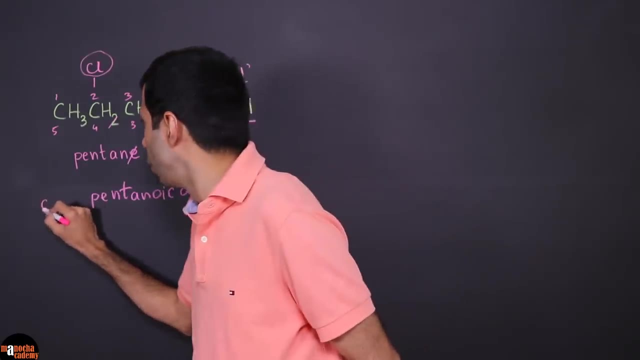 So what will the name of this compound be? So it's basically a pentanoic acid And the halogen comes in the prefix, So it would be a chloropentanoic acid. But we need to do the numbering. 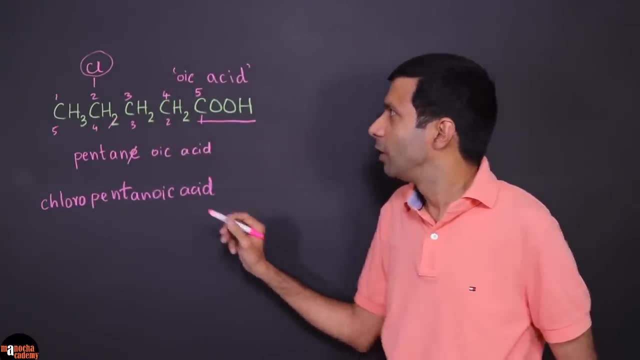 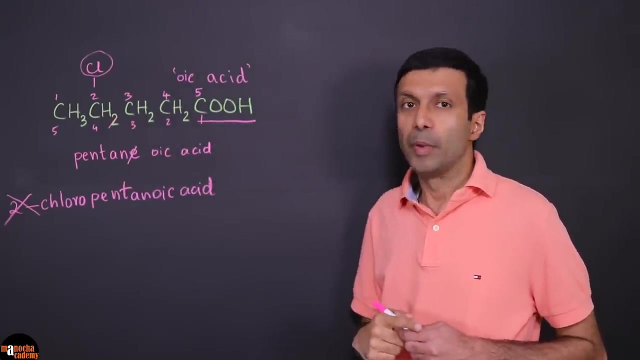 Right. So what number should we choose? If we look at the smallest number, we will think of writing as 2-chloropentanoic acid. But that's the wrong answer. Let me explain you why. Because in this compound. 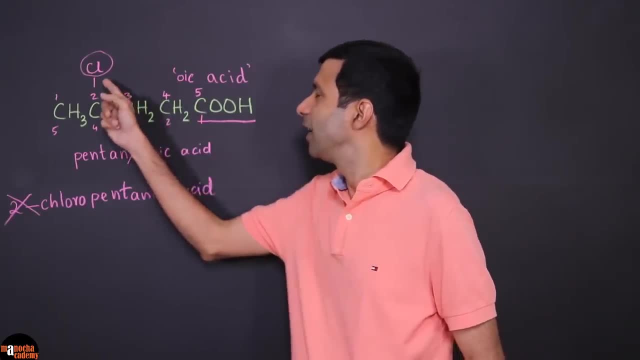 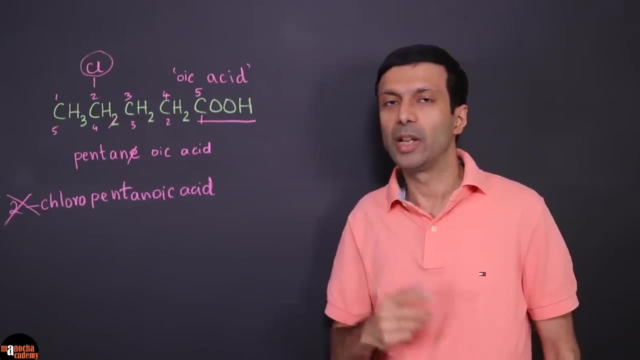 can you see that there are two functional groups, An acid and a halogen, And then there's an important priority order that we need to follow. So let me write down the priority list here. So what is the priority list that you need to know? 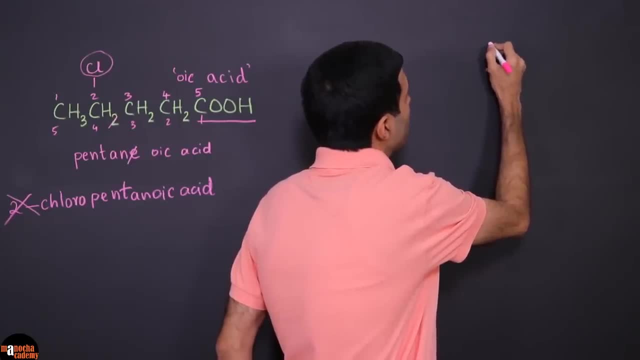 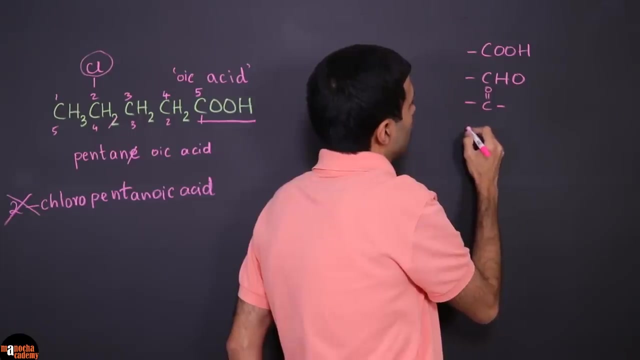 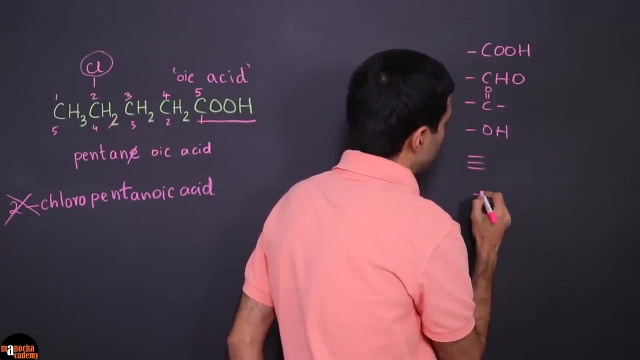 So we have on the top priority. we have the acids, So that's COH, Then we have aldehydes, Followed by ketones, Then alcohols, Then you have the triple bond, Double bond, Okay. 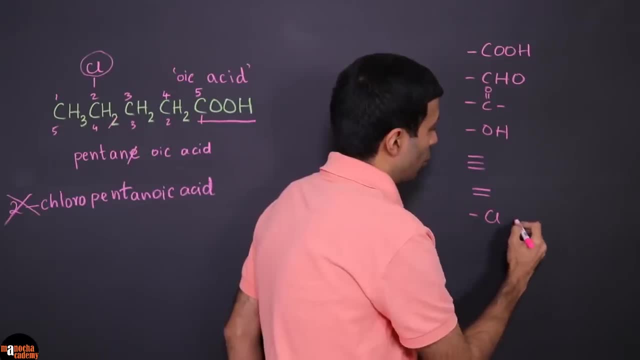 And then you have the halogens, So things like chloro, bromo, Right. And then you have the alkynes, So things like methyl ethyl. So these are the highest priority. So this is our priority list here. 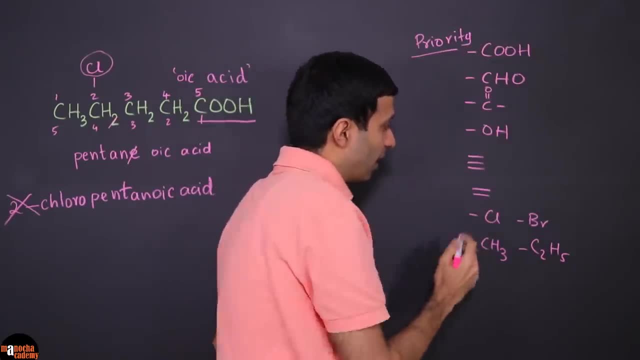 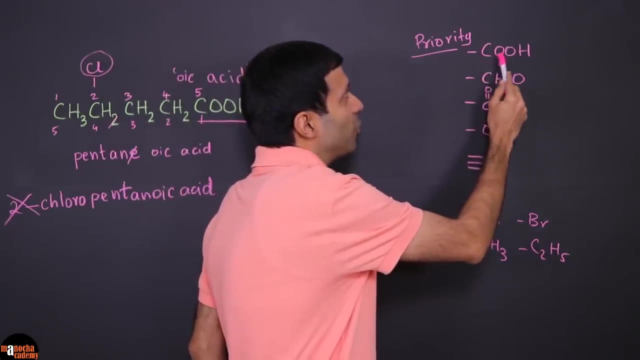 And the top ones are at higher priority than the, And this one is at the lowest priority. An easy way to remember is this one has the most atoms: One, two, three, four. So that's the top priority here. 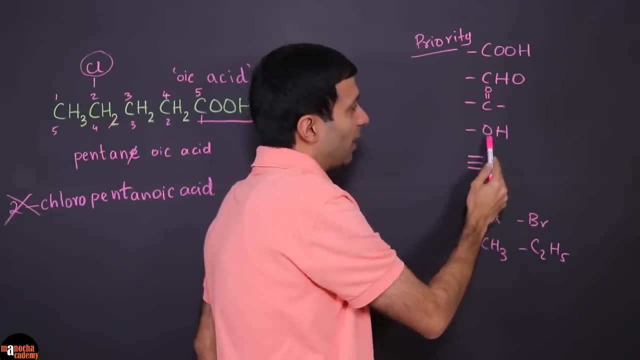 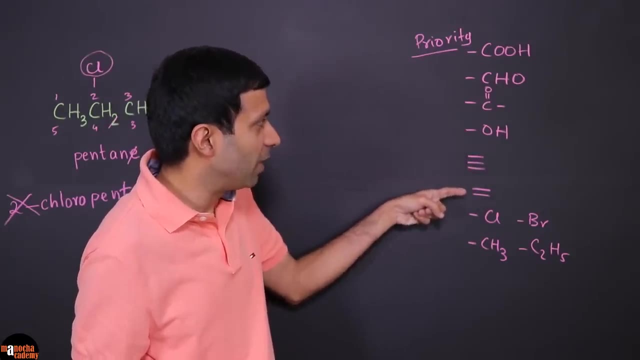 This has three, This has two, And this one doesn't have carbon. And you know, in organic chemistry carbon is the king, So that's alcohol. Then you have the triple and double bond, Followed by this functional group of halogens. 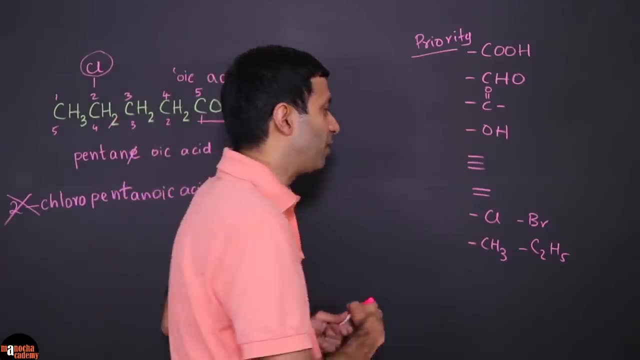 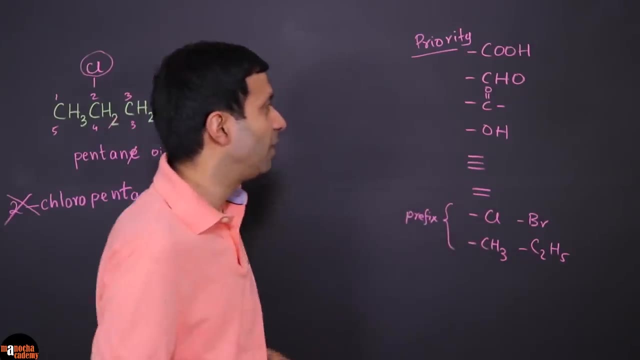 And then the alkynes, And remember these guys were added as prefix in the name. So the prefix fellows come down at the priority list And all of these affect the suffix of the name. So you can note down this important priority list. 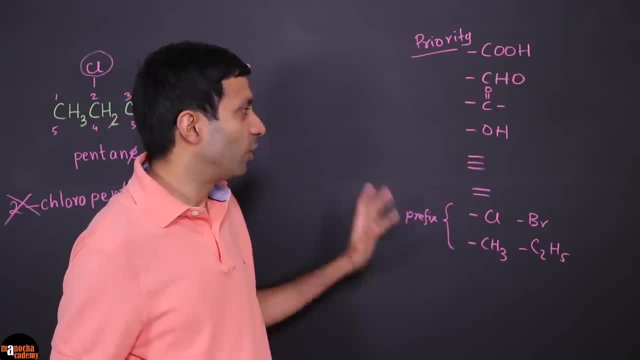 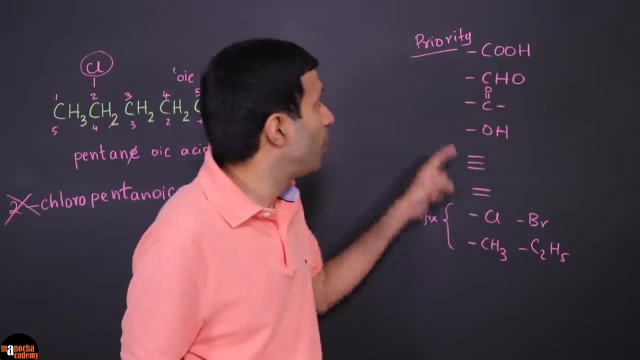 And the numbering will be based on that. So let's apply this for our compound here. So we have acid and a halogen. So according to our priority list, acid gets the top priority. So he wants position number one. 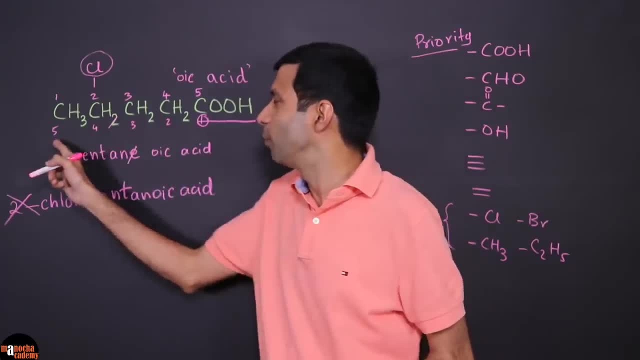 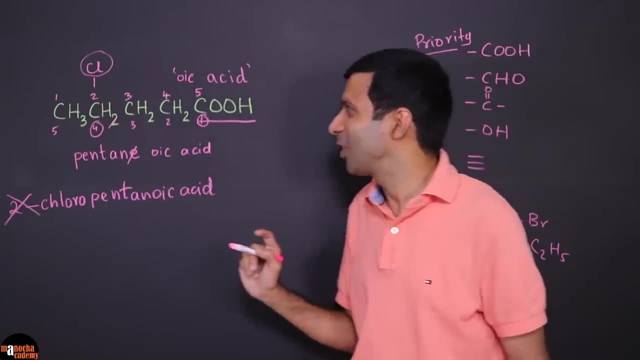 Right. So we need to follow this numbering scheme, not this one, And the halogen is at position four. So, basically, what is this compound? It's a 4-chloropentane-1-oic acid, Right? 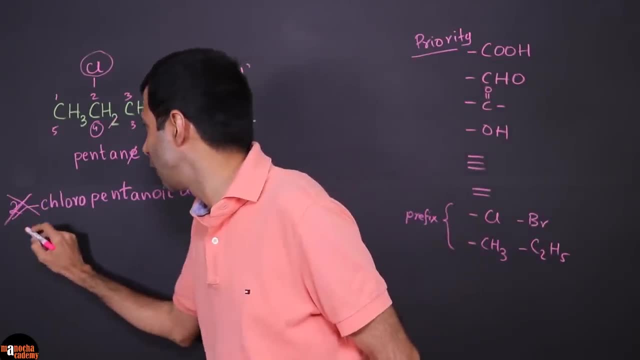 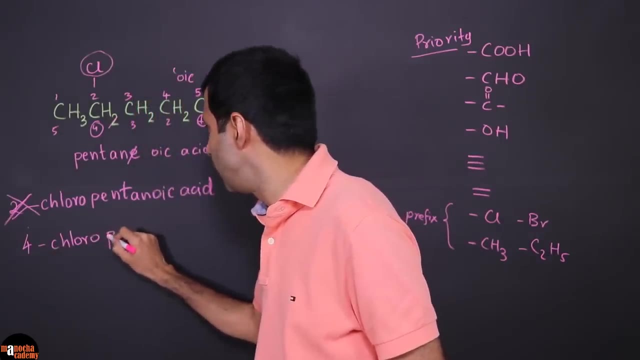 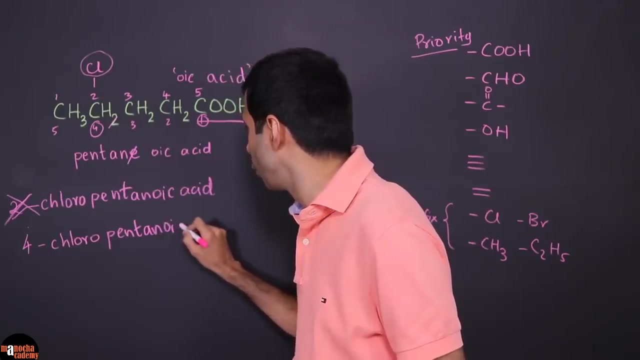 So we can simply write that as instead of a 2-chloro, it's going to be a 4-chloro Right Pentane. But I won't write 1 because it's not needed, So it will just be 4-chloropentanoic acid. 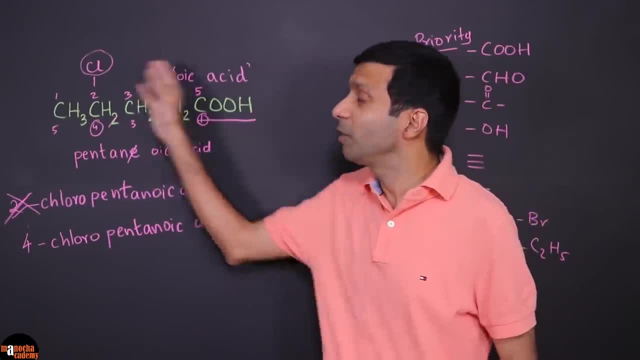 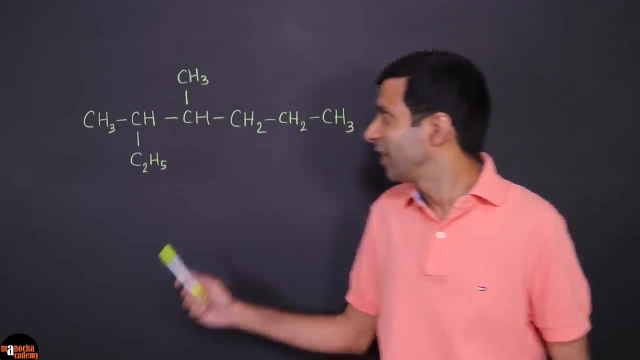 So this is an important thing. we've learned That when there are multiple functional groups, we need to apply a priority list to determine the numbering here. Here's another example for you. Why don't you pause the video and try writing the IUPAC name? 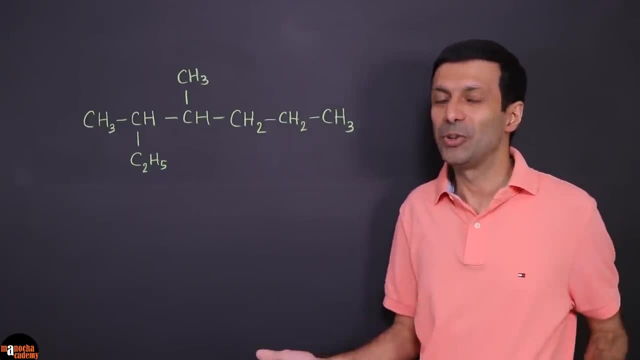 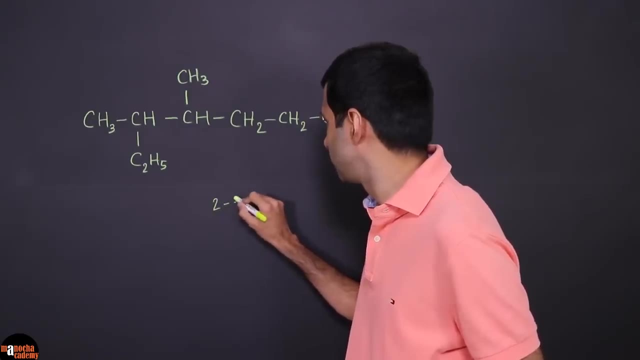 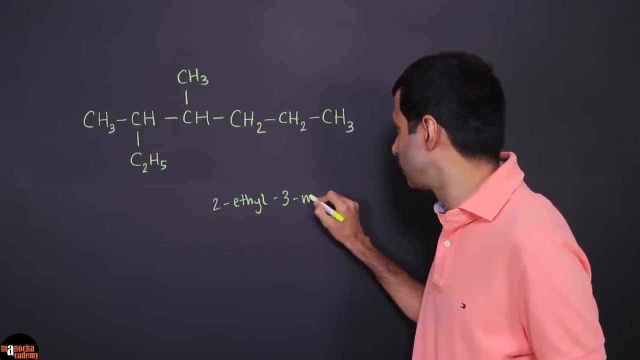 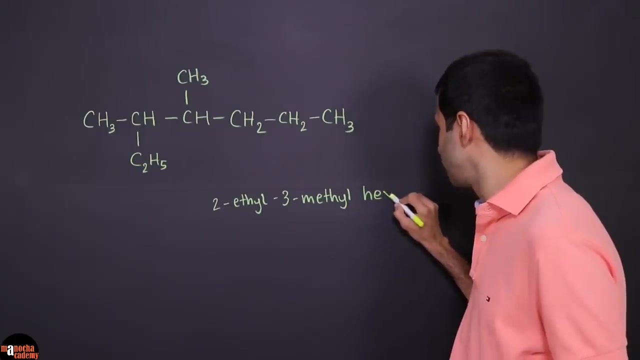 yourself for this one. So what is the answer you got? Is it 2-ethyl and 3-methyl, 1,, 2,, 3,, 4,, 5, 6 hexane? So is this your answer? 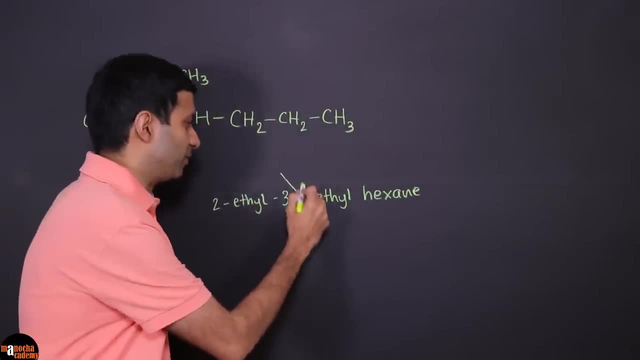 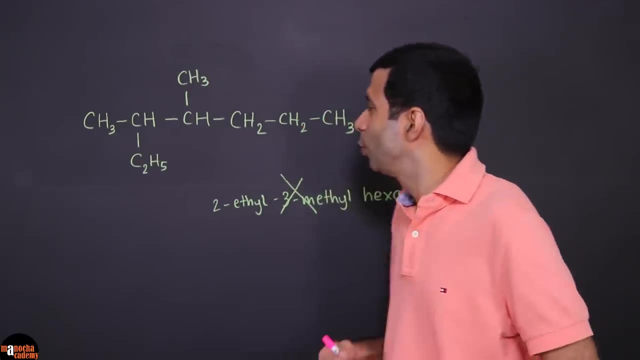 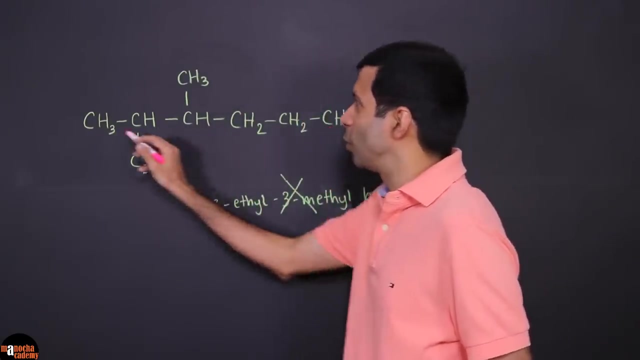 Actually, this answer is wrong. So what is the right answer here? Let's take a closer look. So if you look carefully, this is not the longest continuous carbon chain. Why? Because this one has 6 carbons. But if you go like this, 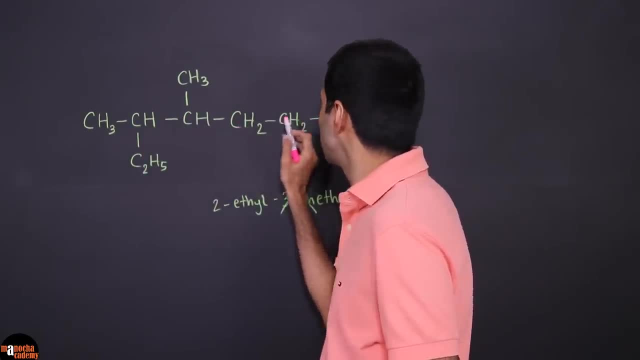 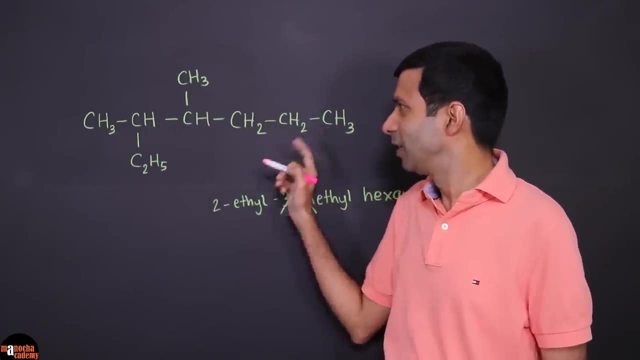 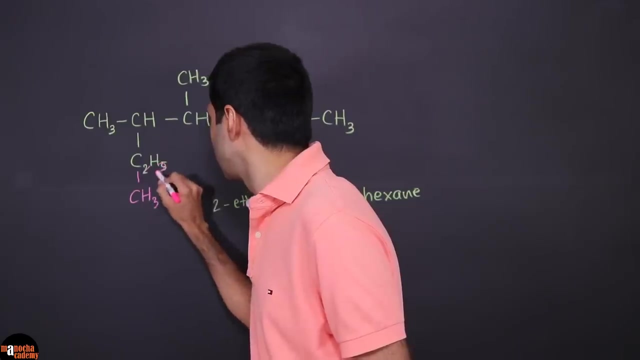 then can you see there will be 2,, 3,, 4,, 5,, 6,, 7 carbons, So the longest continuous carbon chain is this one. So it's easier if we expand this one and write it as: 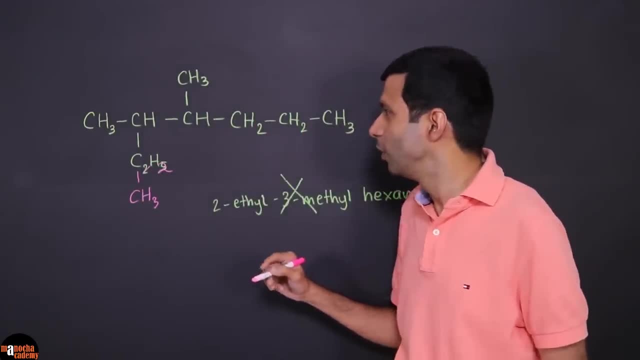 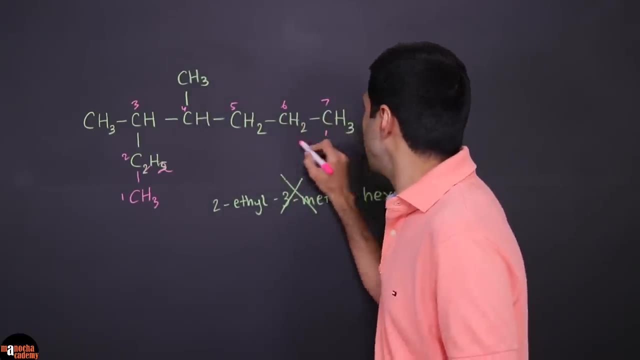 Right. So I just expanded the ethyl there for you, And let's number our longest carbon chain here, So 4, 5,, 6,, 7.. And again backwards: 1, 2,, 3,, 4,, 5,, 6,, 7.. 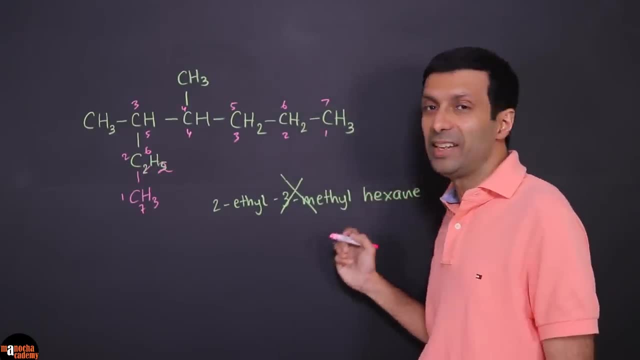 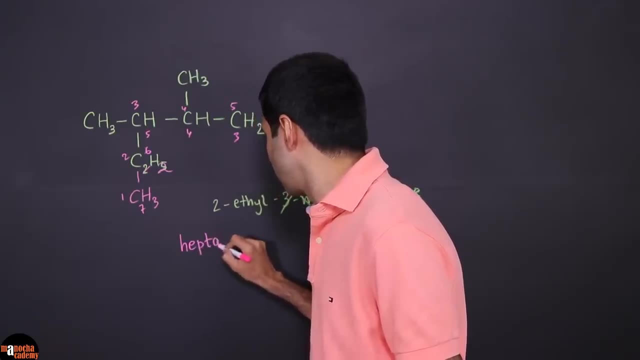 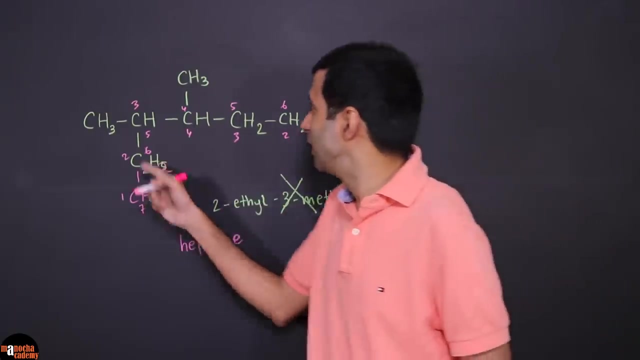 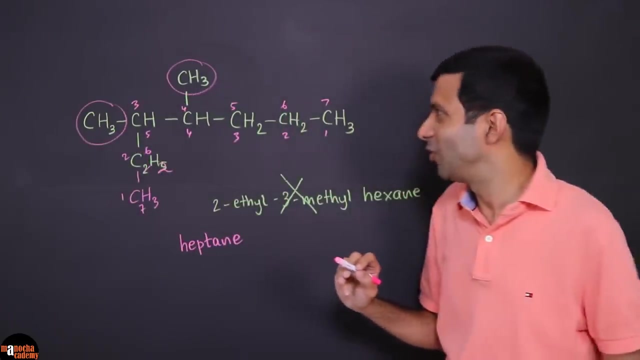 Right. So this is not basically a hexane, It's a heptane Right. And what are the attachments in front of this name? Because you can see the attachments or the substituents we have? here are 2 CH3s. 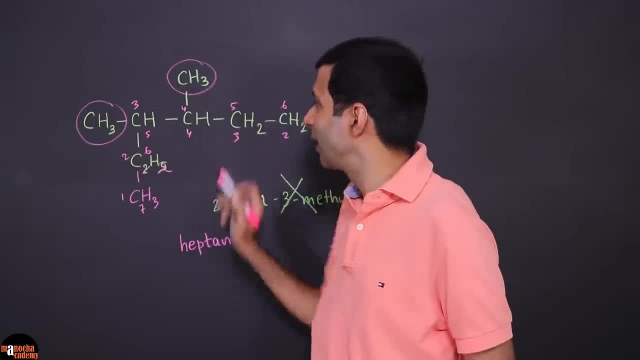 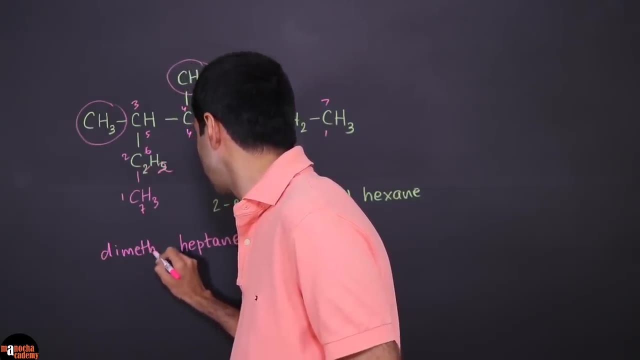 Right. So that's basically, And you know, CH3 is the alkyl group, So it's a dimethyl. So we have a dimethyl in front of the name here, the prefix part, And what are its positions? 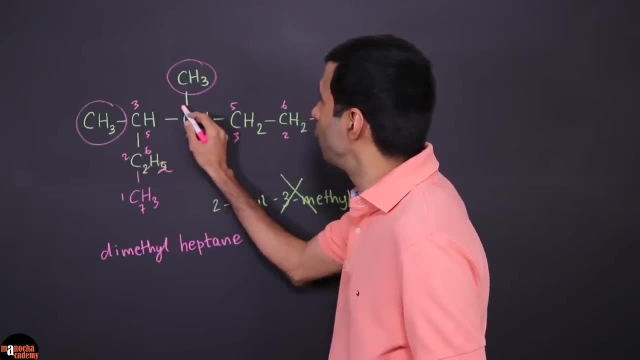 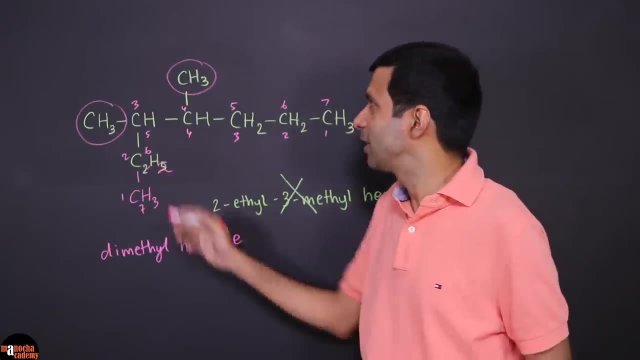 It's at position 1,, 2,, 3, and 4. if we number this way, So 3 and 4 here, And if we go this way, it's at 4 and 5.. So again, we'll choose the smallest number. 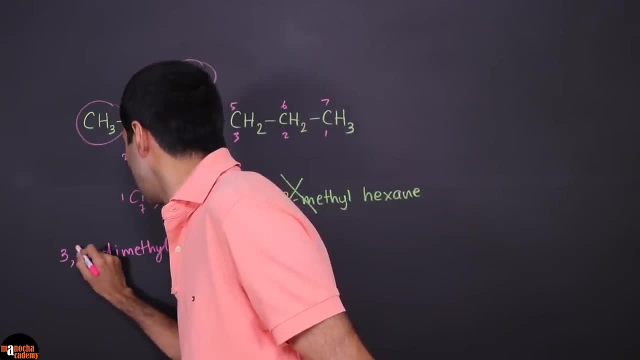 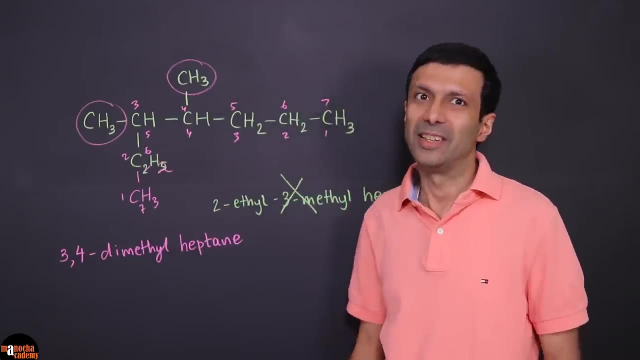 which is 3 and 4.. So the name is going to be 3, 4 dimethyl heptane. So that's our correct answer here. Okay, let's try this one now. Here we have 4 carbons. 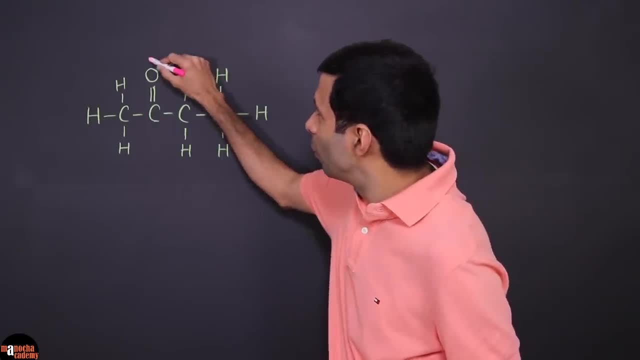 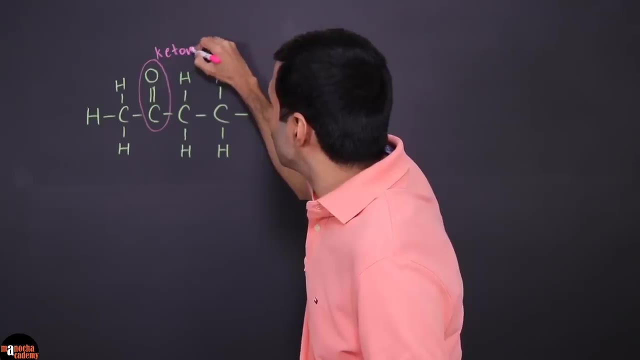 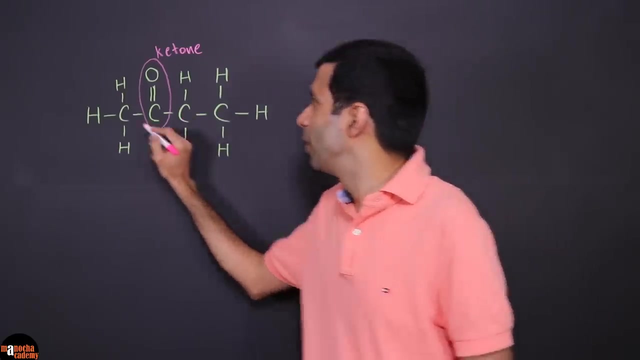 And can you see the functional group here? What is the functional group? That's right, It's a ketone, Because you have C double bond, O and carbon on both sides. Right, So let's number our longest carbon chain: 1,, 2,, 3,, 4.. 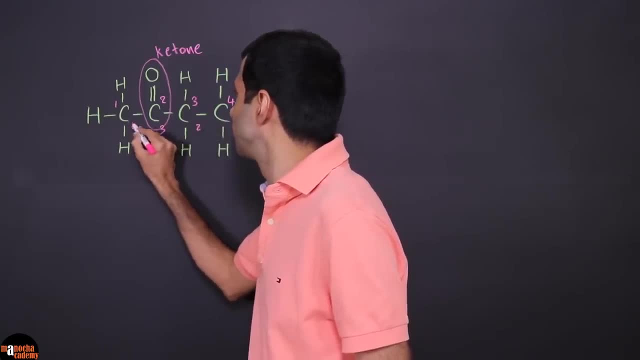 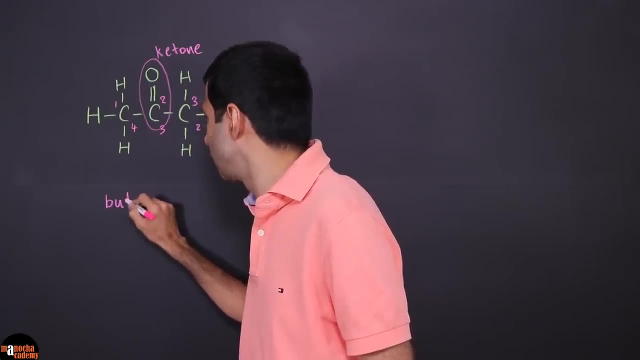 And reverse 1,, 2,, 3,, 4.. Okay, So if we ignore the functional group, it would have been a butane, Right, But there's a functional group in there, So I'm going to delete the E. 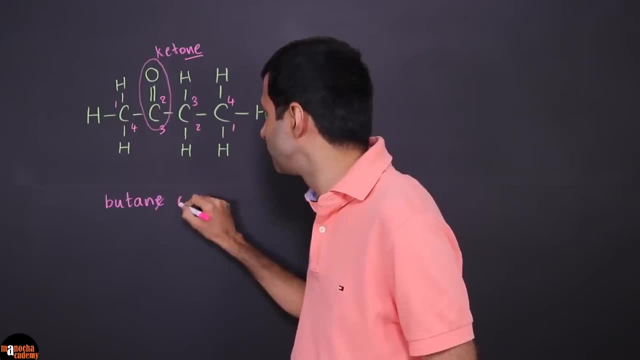 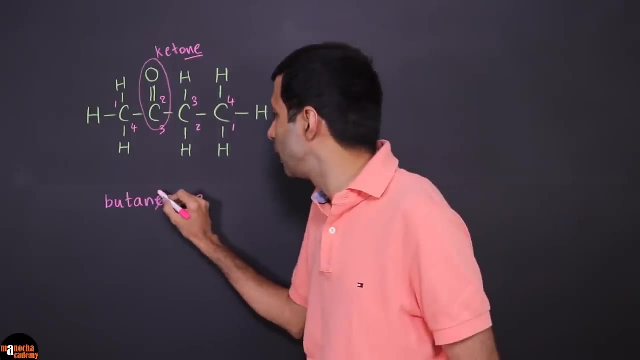 And you know, in ketone the O gets added, So it becomes a butanone. And what is the position of the functional group? It's at position 2.. So that would be make it a butane 2-one. 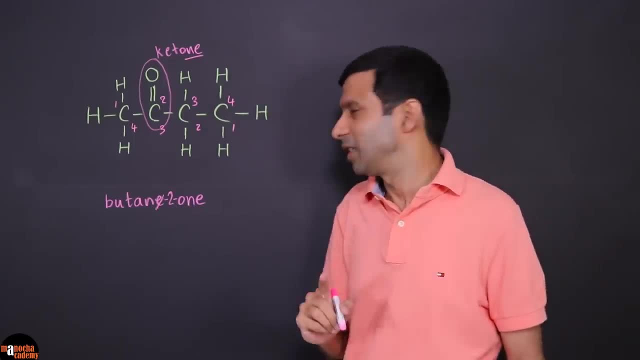 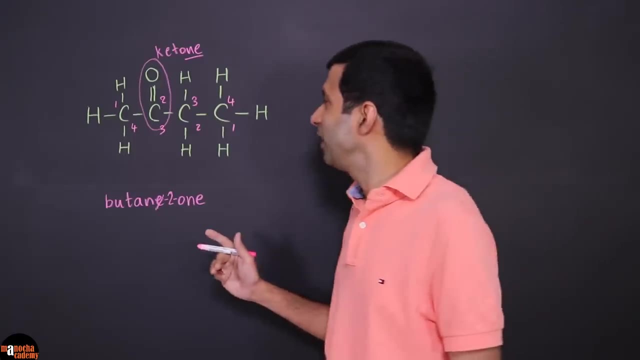 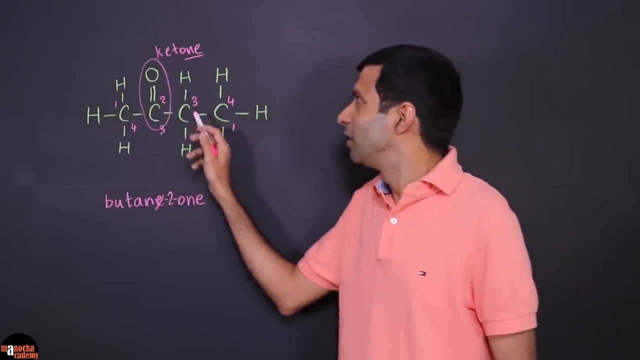 Right, But there's something interesting here. If you write this name, it's probably fine, But strictly speaking, if you look here, if I shift the double bond over here, then what will the name be? It's not going to be butane 3-one.